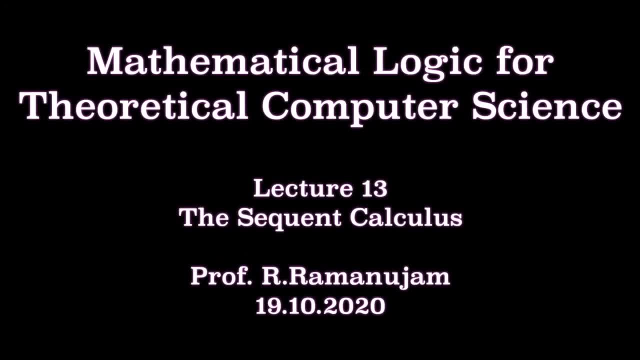 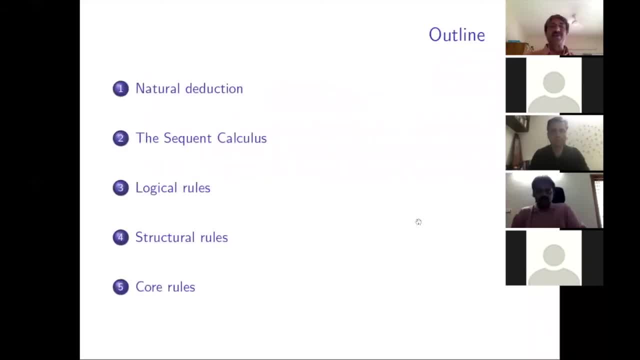 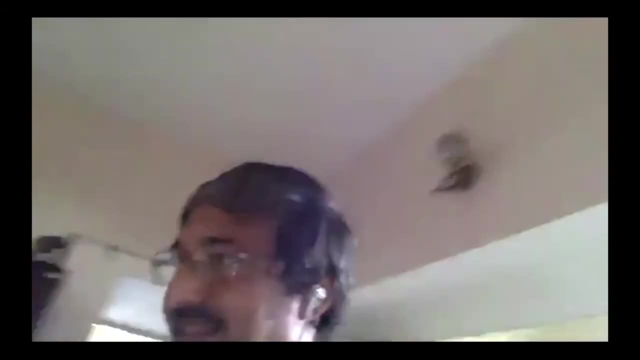 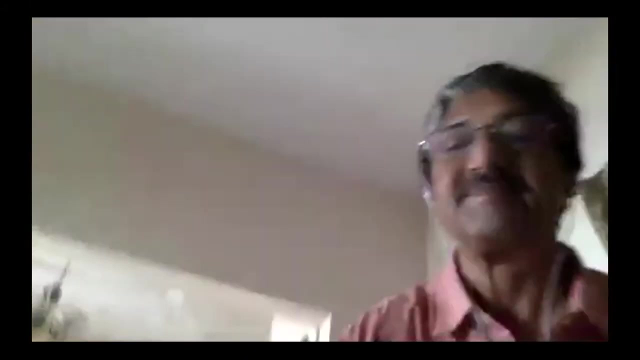 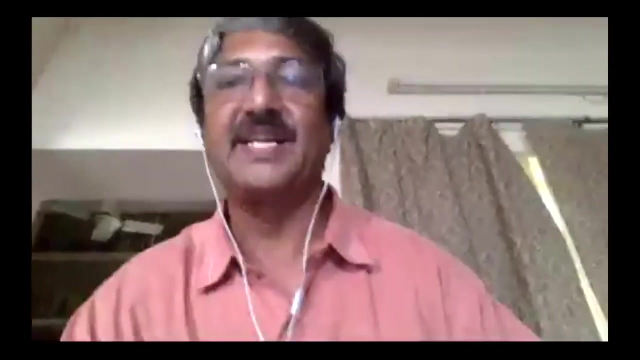 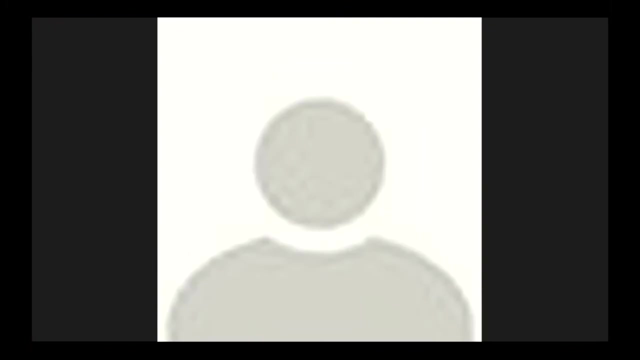 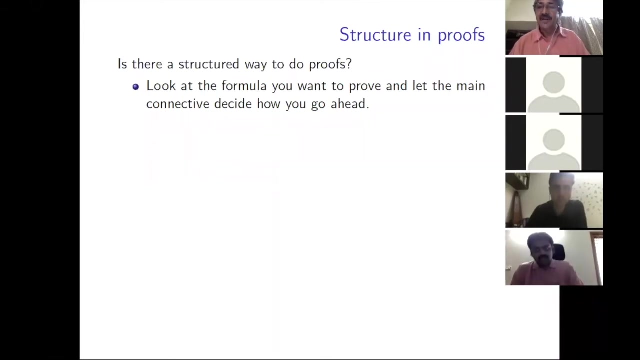 Yeah, so we are introducing the sequence calculus, and first let me do a natural deduction, a recap of natural deduction, which is what we talked about. So the main idea is that internet is not coming there. I'll try from here, Then we can't hear you. 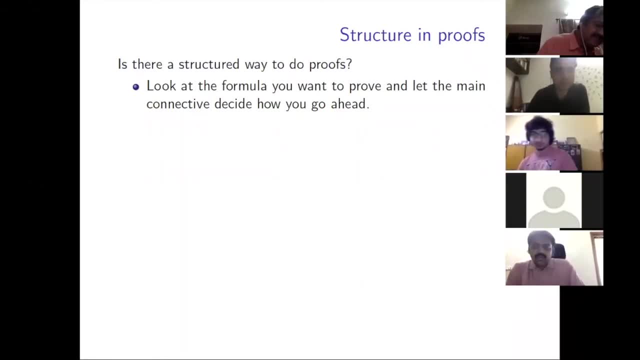 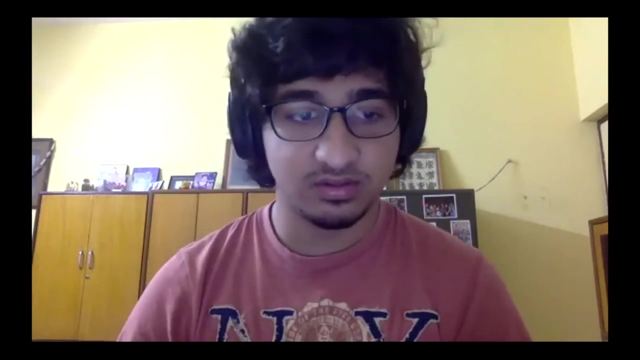 What about now? Can you hear me? Yes, now I can, And the screen is okay. Yes, sir, Okay. So yeah, Again. not able to hear you, sir, Again, So maybe you could turn off your video. 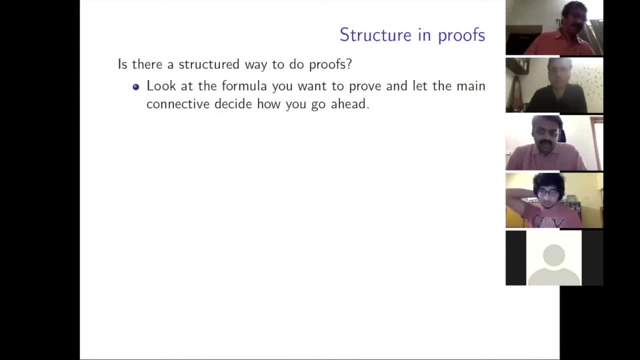 You're not audible, sir, So you're not audible, Okay, Okay, What about now? Yes, yes, sir, And is the screen moving, or is it stuck? Yeah, yeah, it's moving, Okay, Yeah, So this is what I said is the spirit of natural deduction. 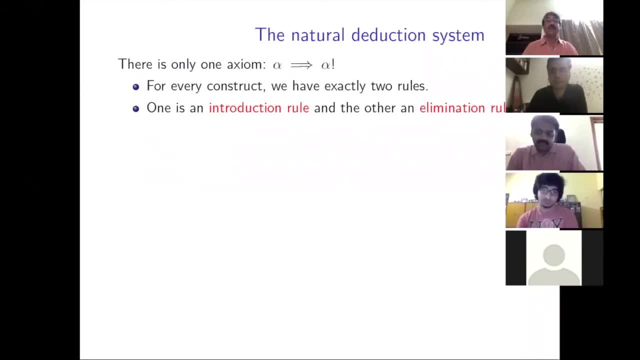 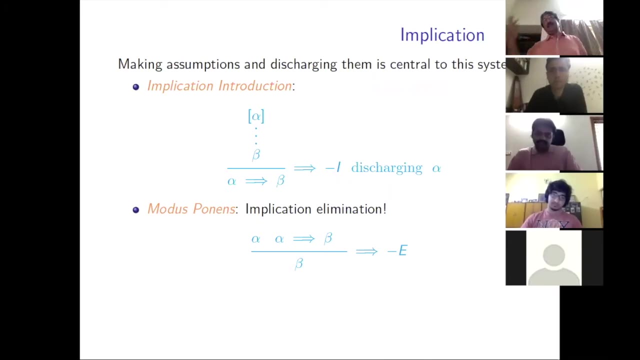 And there's only one axiom: alpha implies alpha And for every construct we have exactly two rules: One is an introduction rule and the other is an elimination rule For implication. the implication introduction is exactly what I just said. You make an assumption- alpha- and from that you go on to beta. 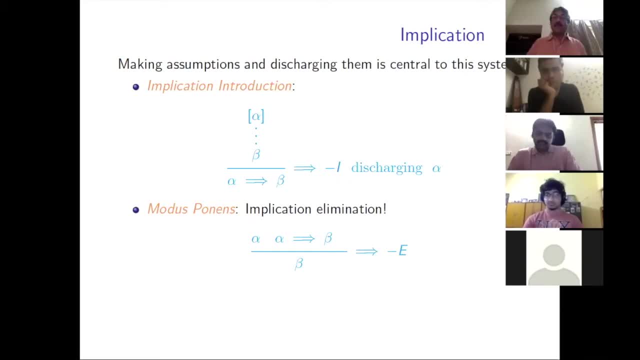 Then you can derive: alpha implies beta where you discharge the assumption. Note that it's very important to nest assumptions. So, for instance, suppose there are two assumptions, There is alpha and assumption, And then there is a beta And then there is a gamma. 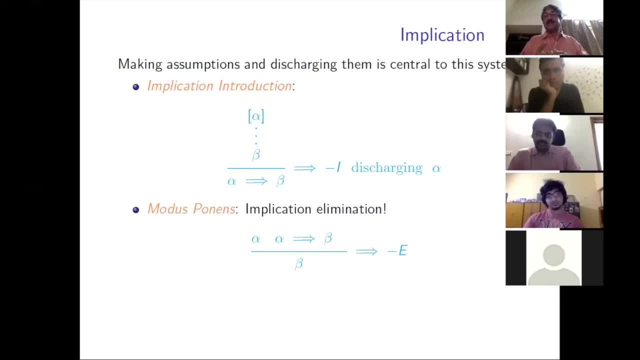 You can't write. alpha implies gamma. It's beta implies gamma, where you discharge beta And then you can discharge alpha by writing. alpha implies beta, implies gamma. So nesting is important, Scope is important, So you have to be careful about that. 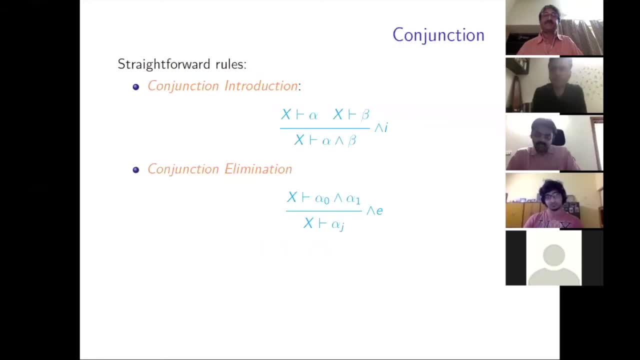 Implication, elimination is exactly more important Then conjunction. this is the natural rules that you think of. If you have derived alpha, if you have derived beta, you can derive alpha and beta. On the other hand, conjunction, elimination is: if you have derived alpha and beta, you can derive alpha and beta. 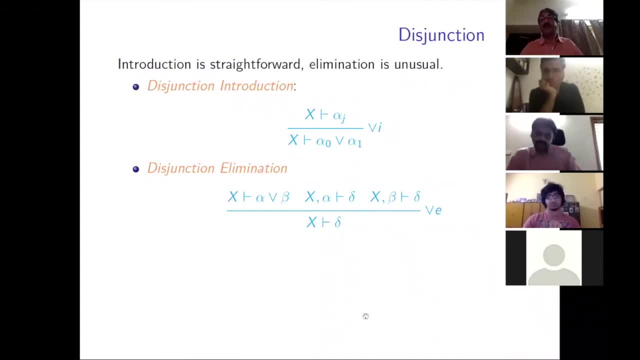 So this junction introduction is straightforward. if you have derived alpha, you can weaken it to alpha or beta. What about elimination? This is what we discussed at length last time. If you have derived, this is case analysis- If you have derived alpha or beta, and assuming alpha, I can derive delta. 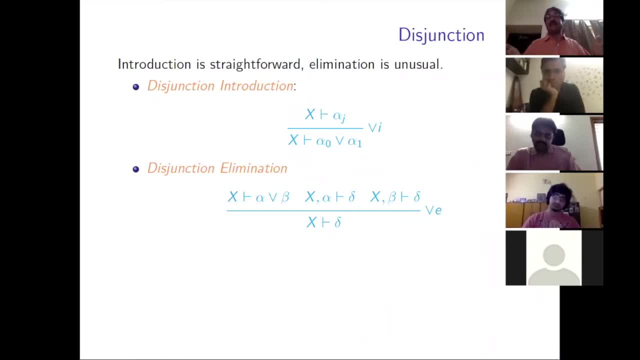 Assuming beta, I can derive delta. In all the cases I have to derive delta. Therefore I can derive delta. So- and this is a very important difference thing- So in natural deduction, disjunction is about case analysis. So, in particular, very often you make the assumption that either this two-order response right- alpha or beta- 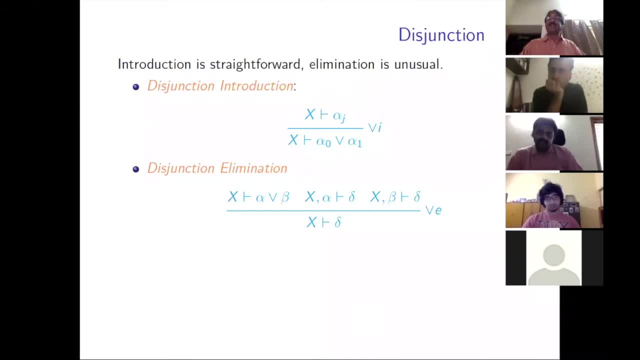 Assuming alpha, I derive delta. Assuming not alpha, I derive delta. In both cases, delta holds therefore delta. This is the way we actually do case analysis And this is again a way, the way in which we state the data. 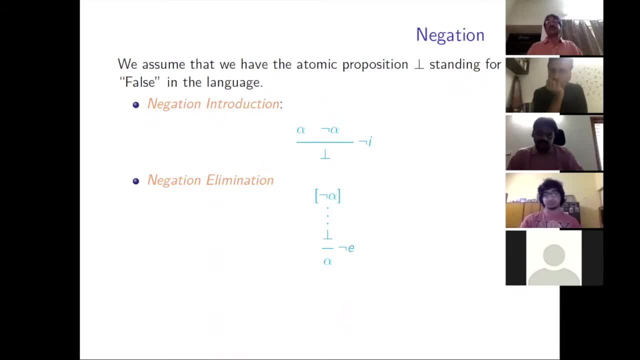 For negation. as I said, I introduced this rule And but if you see the literature, there are different forms of negation and deduction. Rightfully, this should be called, You know, false introduction and false introduction. From a contradiction you derive false. 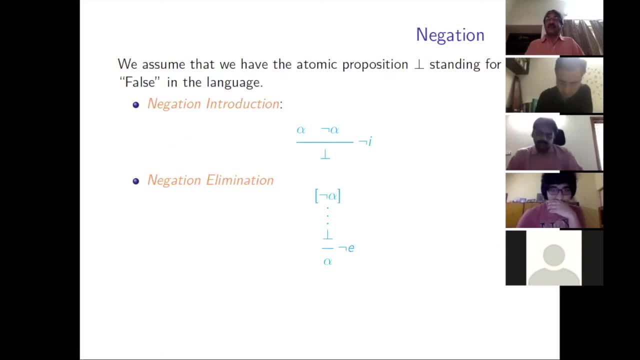 And assuming negation alpha. if you have derived false, come back. But, as I said, there are different versions of, So today I'm going to. So this is one proof system And, like I said, you can prove that natural deduction is complete. 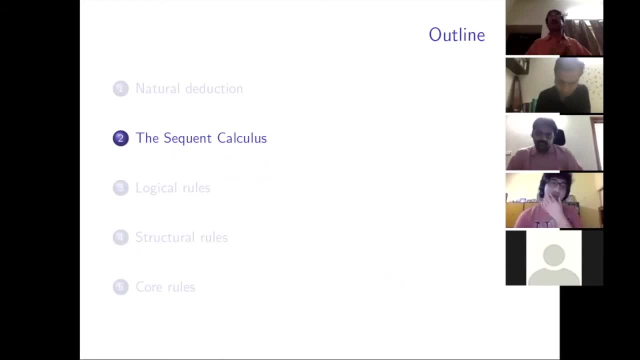 By showing that all the rules of natural deduction actually Derivable in the Hilbert system. That's something very straightforward. Try it out And once you have them derived in the Hilbert system. Therefore, it means that whenever a formula is valid, 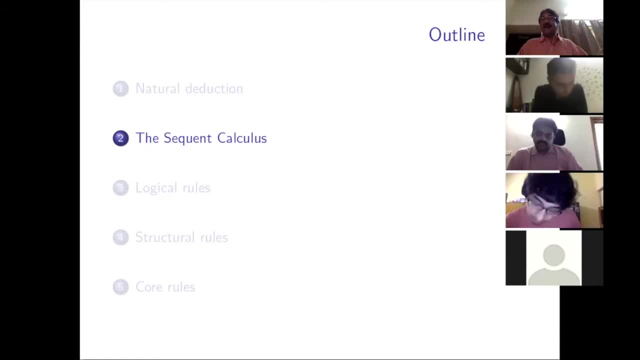 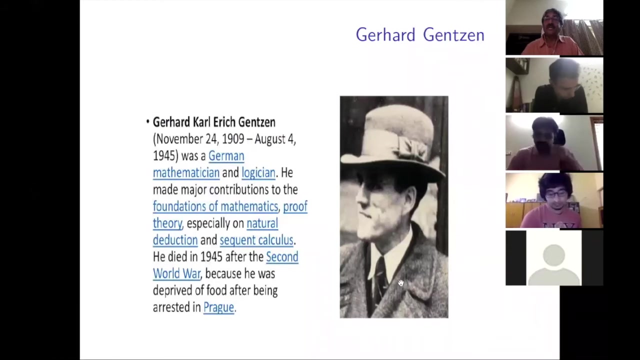 We already know that there is a proof in the Hilbert system And now you can derive. Yeah, So you can all. basically, And now to sequent calculus. This is both natural deduction and sequent calculus, defined by Gerhard Jensen. 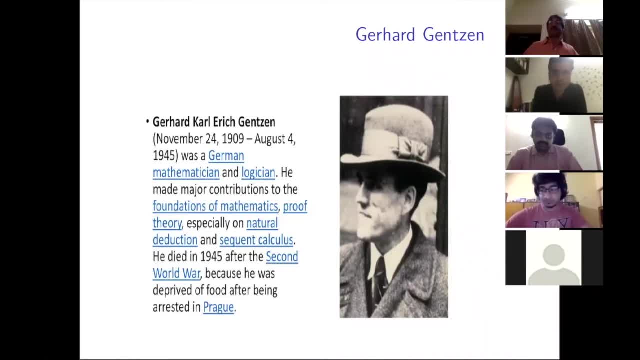 Gerhard Jensen was born in 1905. He died in 1935.. He made major contributions to the foundations of natural deduction, And especially natural deduction and sequent calculus. He died in 1945.. Immediately after the Second World War. 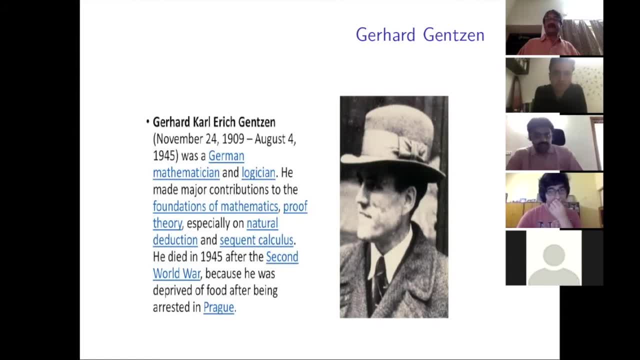 And he was arrested in Prague And So he was all of 36 years old And he wrote landmark papers in 1934 and 1935.. Those years, you know, 1931 was Gerhard's paper, 1934 and 1935 were Jensen's papers. 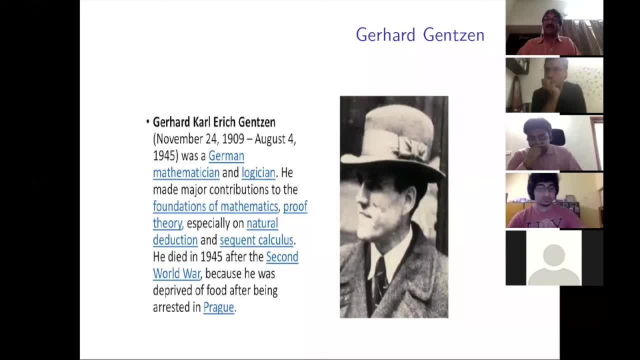 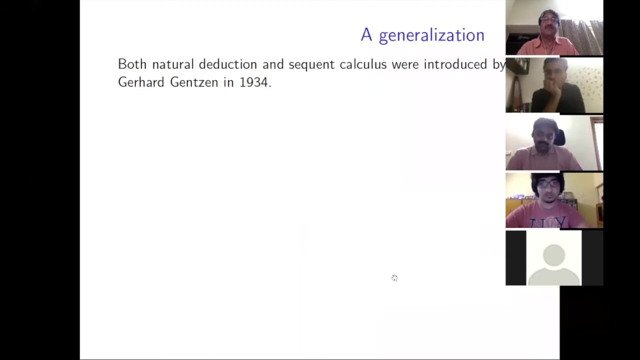 1936 was Turing's. These were the years where mathematical logic was unbound. So if Gerhard's paper in 1931 founded, I call it the beginning of mathematical logic And Jensen's paper was the beginning of. So they were both introduced by Jensen in 1934. 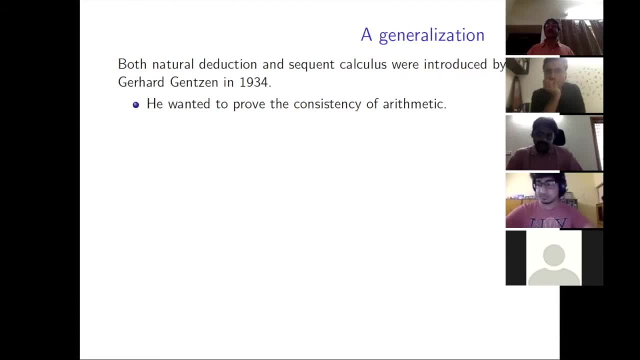 And his main interest was in proving the consistency of. Now Hilbert had proved the consistency of geometry And in fact that was his PhD thesis And that was where he actually showed that Riemannian geometry was actually consistent. And this was very important because, after the Euclid's Parallel Postulate, 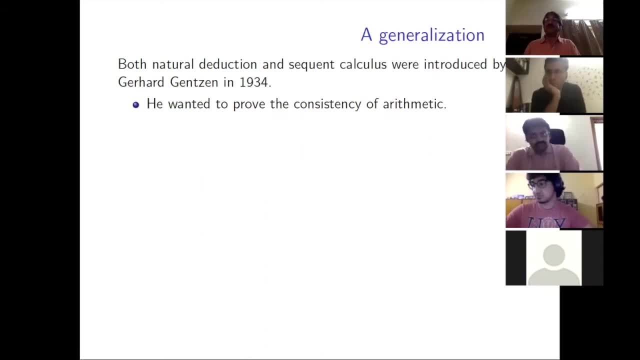 it was clear that these were independent. There was non-Euclidean geometry around, But how do you show that it was consistent? And Hilbert did this And, along with Bernays, wrote his own foundations of geometry. The question was arithmetic. 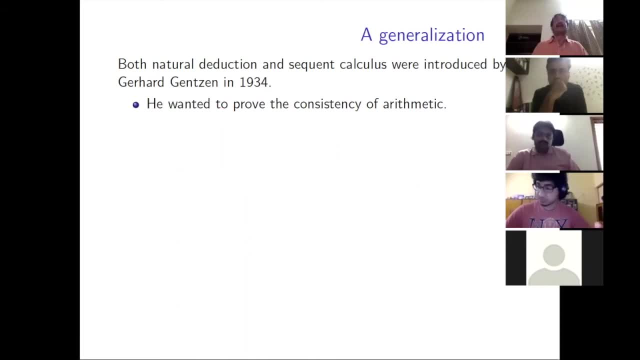 How do you prove the consistency of geometry? And this was a major project And Jensen wanted to take it up. He tried with natural deduction And his whole idea of formalization of natural deduction was to solve mathematicians' new proofs. But he couldn't do it. 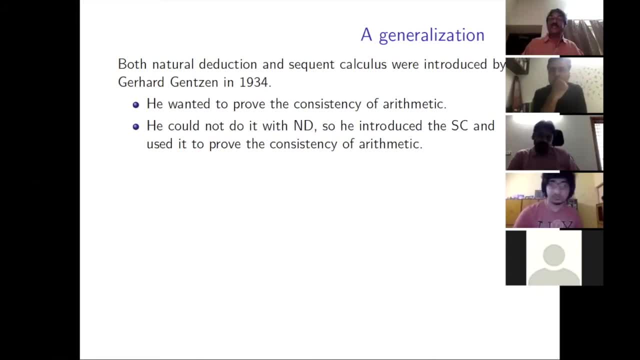 And therefore he introduced a secret calculus and used it to prove consistency of arithmetic. And his proof of consistency of arithmetic and that ordinal epsilon naughts is one of the most beautiful landmark results of mathematical logic. We won't be able to do that proof here. 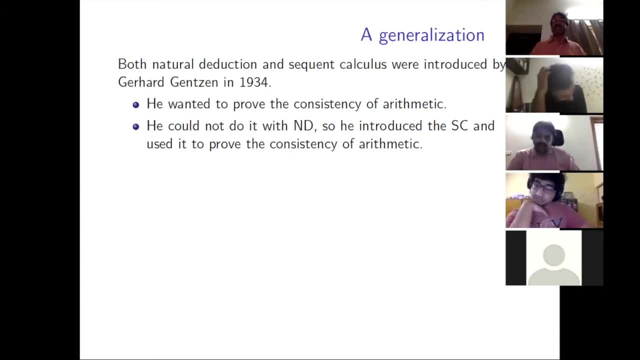 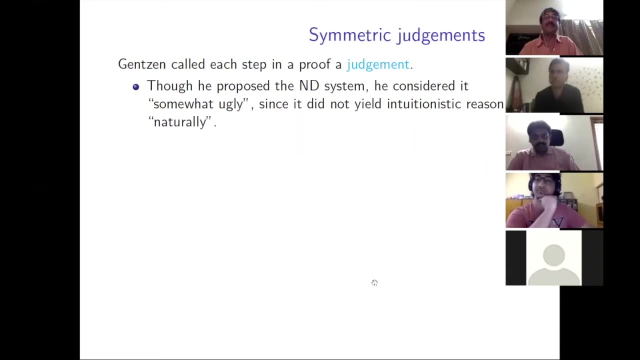 But I hope I'll at least do some bit of consistency of system that even that will take up. I would say it's become the most cherished tool of this year And you will see why It's really beautiful. So for Jensen, each step in a proof is a judgment. 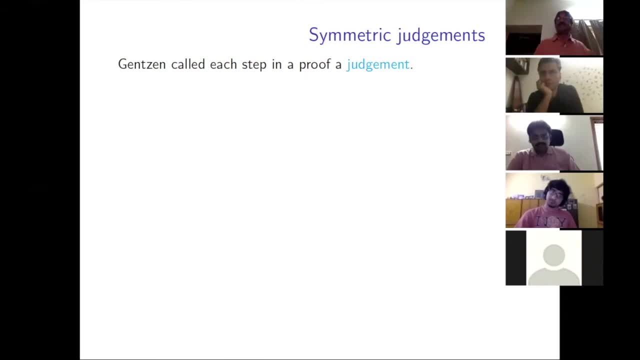 When you write down a statement, you are making a judgment, And so for him, this idea that from passage from assumptions to conclusions is not, like in the Hilbert case, the entire proof or existence of a proof, But every step is actually a passage from assumptions to conclusions. 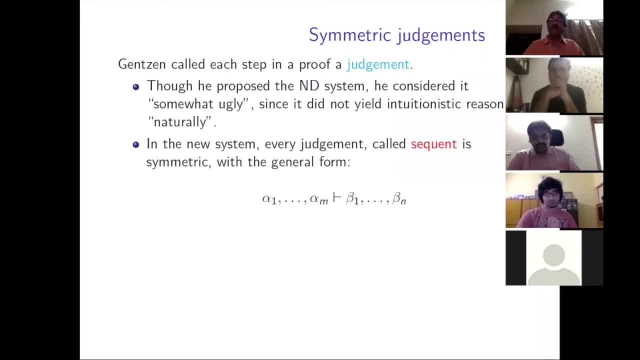 So, though he proposed the natural deduction system, he considered it somewhat ugly Since it for of course. one important reason for him was: you know, if you look at reductio ad absurdum, they're doing something weird. 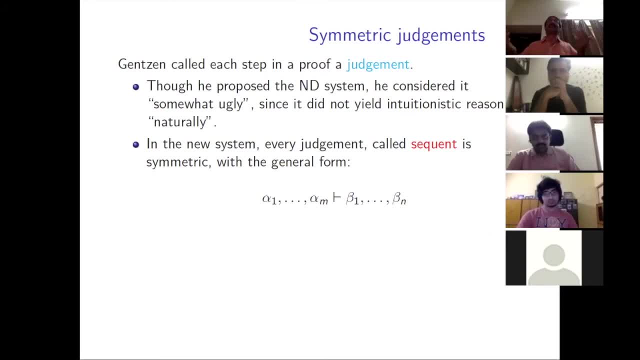 I mean it's theoretically. the rules for AND and OR are not symmetric, They're not dual And the proof rules are asymmetric. In a rule you make you have, there are a lot, several premises, but only one conclusion. 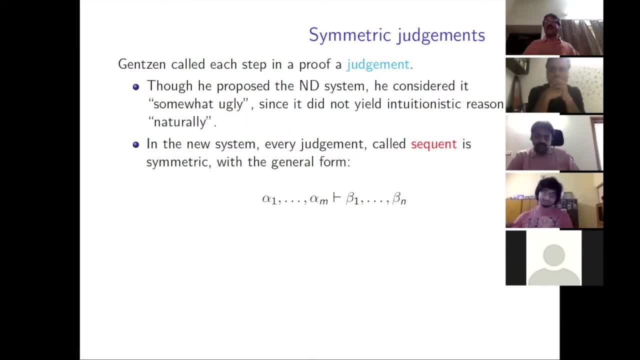 Right. So, and you take the tree shape very literally, The idea of proof rules, with many premises, and one conclusion Gives rise to a tree Proof tree. And Jensen was questioning that. Why shouldn't it be a graph? I mean, why should it be a proof net? 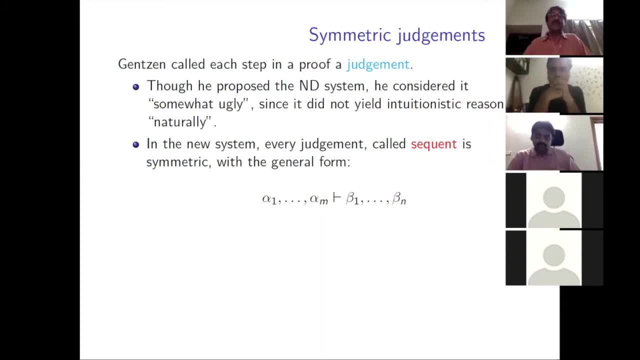 This is what you model in positions. So, and an important thing for him was also the intuitionistic logic, which doesn't come out naturally, I must say. it's not as ugly as it says, but in any case, In any case. 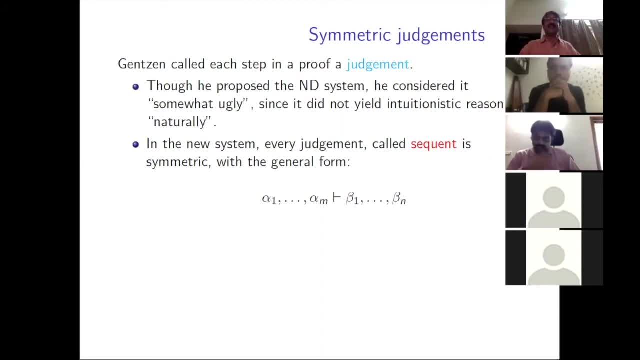 Jensen was really after symmetry He. so in the new system every judgment or the sequence is symmetry And the general form is that you have a sequence of assumptions and you have a sequence of conclusions. So this is the idea of a judgment. 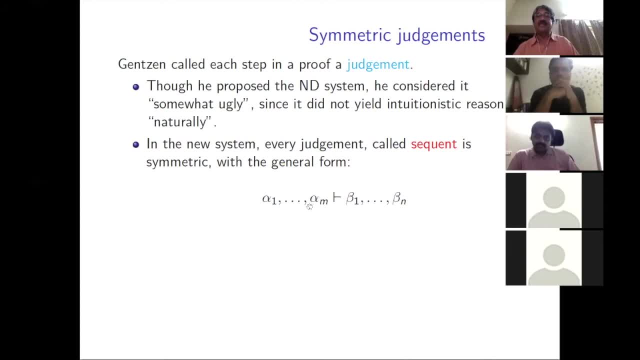 Right. So think of these. So now, from these premises, alpha one through alpha n- you derive a conclusion: beta one through beta n. And the way to read it, the interpretation, is that the conjunction of all the formulas on the left hand side implies: 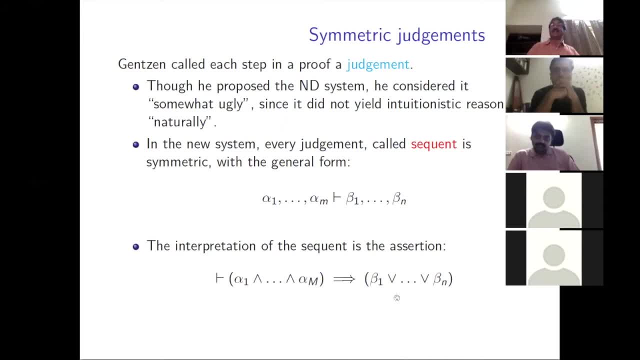 the disjunction of all the formulas on the left hand side. What you're saying is that if I assume that alpha one through alpha n hold, then I can get a beta one, I can get a beta two. So the disjunction of all of them is something like that. 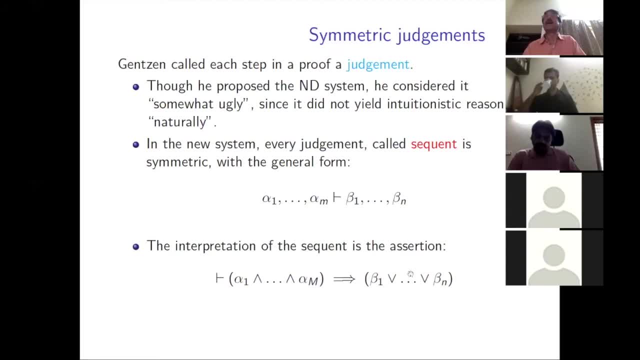 So this is the fundamental idea of a sequence, And the sequence calculus is to manipulate sequence. So how do you derive one sequence from another? That's that. So it's very close to natural deduction. But this very important distinction and, as you will see, 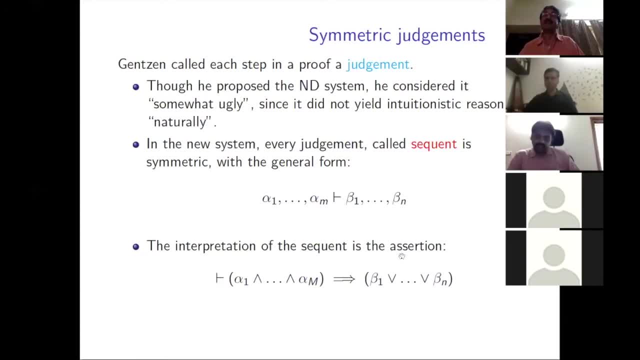 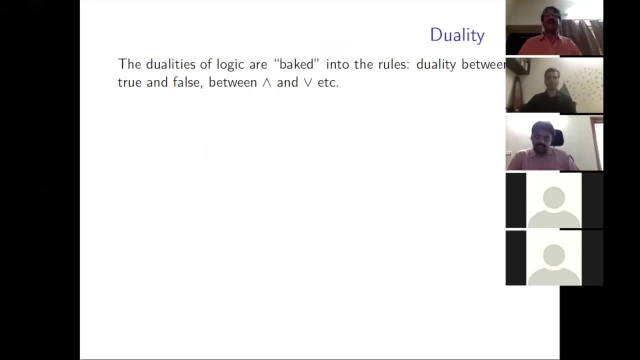 it's almost a fanatical devotion to symmetry and logic. So the dualities of logic are baked into this. So the duality between true and false, between conjunction and disjunction, are all the same. So you don't, you know? 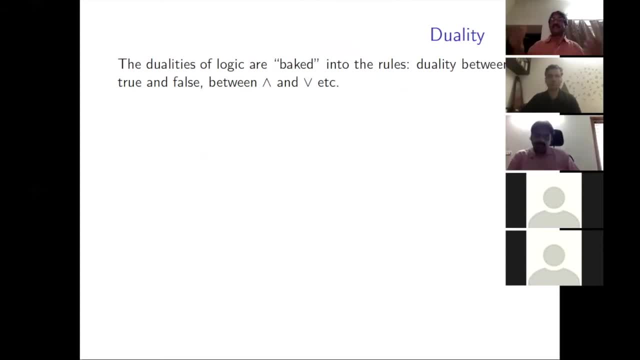 like I said, in natural deduction, conjunction introduction and conjunction elimination are completely straightforward. If you take the dual thing, disjunction introduction is straightforward but disjunction elimination is not. That will give you an example of that. There's a lot more that's mentioned. 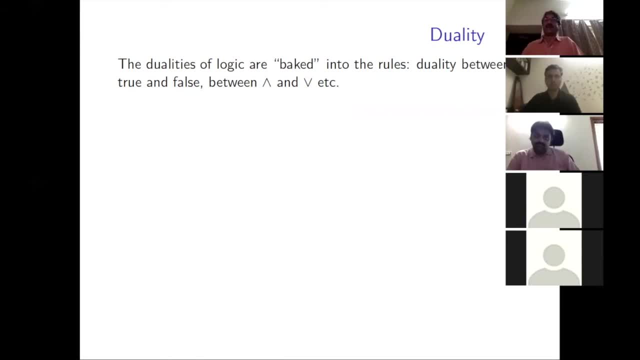 And negation, for instance, is treated in a very strange way. So all that is something that gets in the way And, as I said, he was wrong. Now for the theory of programming languages. there is a very strong computational interpretation of symmetry calculus. 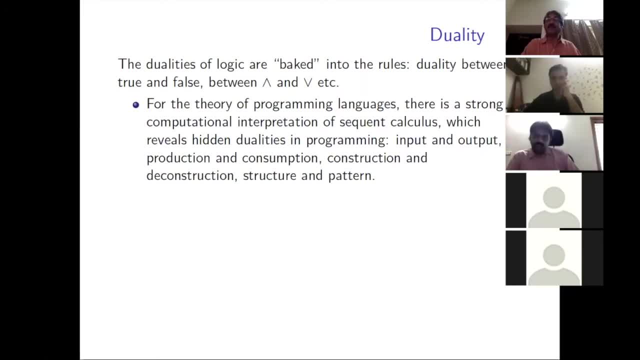 which actually reveals hidden dualities in programming And for instance, the input-output duality, you know, reversing computations in one direction, production and consumption of resources, construction and deconstruction of structure and pattern. So usually when I do, 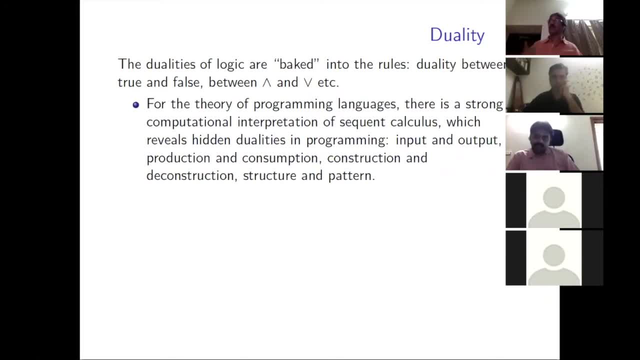 when I teach a programming language theory course, I actually show the connection between these features, typed by that intuitionistic logic, and these computational interpretations I've seen. But it's something that's important And it's a thing that is gone many years since we talked. 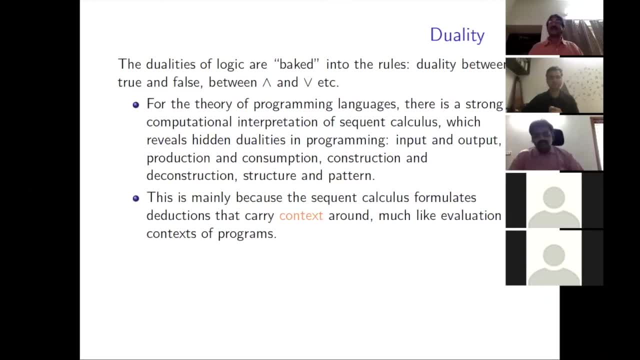 I'm interested in these things But semantics of programming languages is a very tight connection, So I'm interested in this. So the mainly because the sequence calculus formulates deductions that carry context around. So this main point is that the idea of only having these sequences around 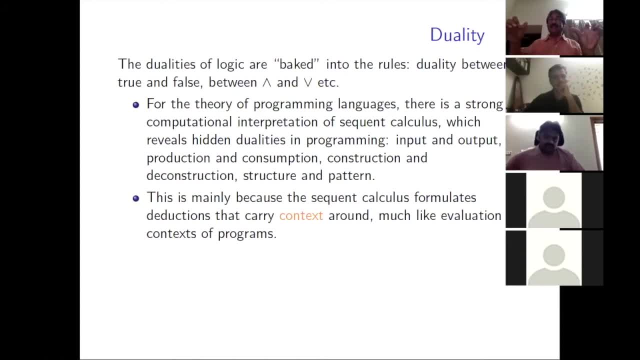 is that these assumptions entail this conclusion, in this context, in the context of some other assumption. So you carry context around and which is much like evaluation context of programs. You've got function programming, function programs and then mutation. Most important thing is carrying context around. 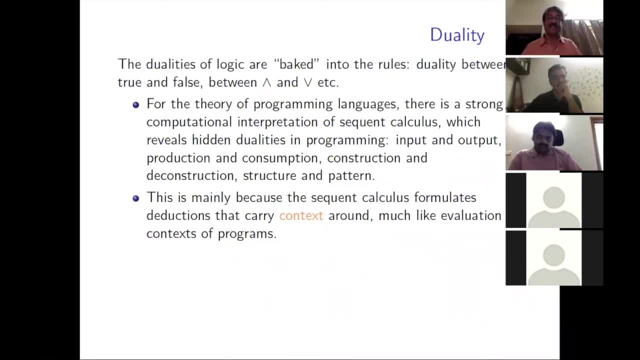 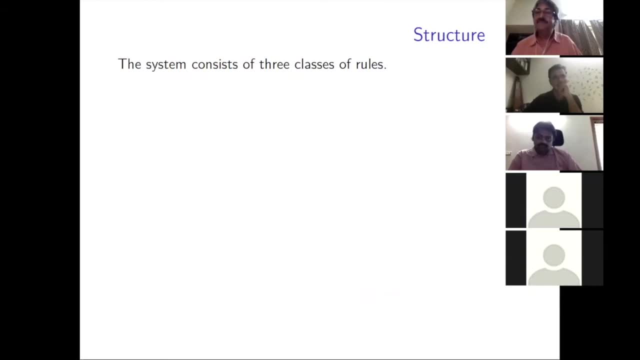 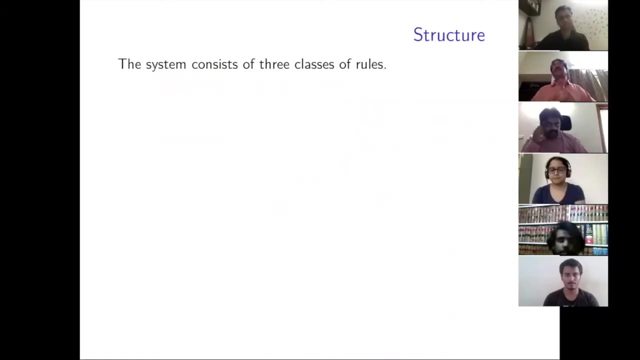 or configurations as state transitions. So anyway, that is Yeah. So what is evaluation context of programs? Well, when you, when you, evaluate a program, or I mean when you run a program, there is one is what is called a program counter. 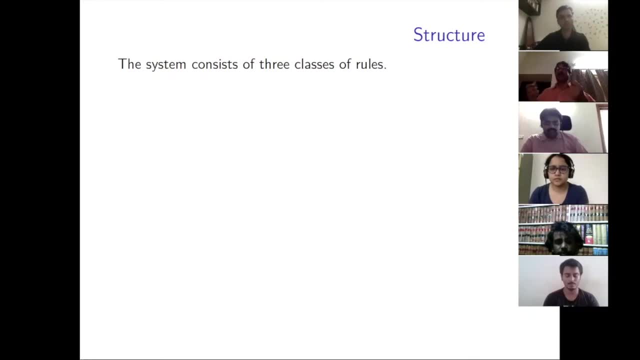 which keeps track of where you are in the program. So that's all And in general, you have a context which tells you what are the values of the global variables, what are the stack, how many which procedures you are running. 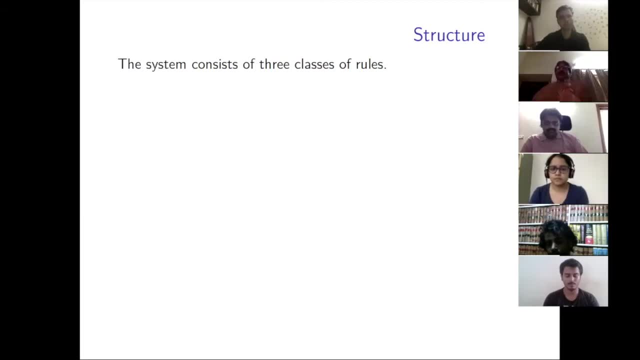 So there is always an evaluation context in which you run And at different contexts the same program statement means very different things, And that's Right. And so if you take the- you know- analogy between computation and deduction very seriously, 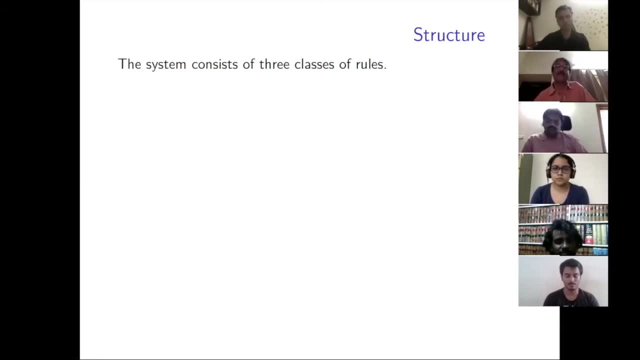 these things actually pan out, Wow. So, Okay, Yeah, Yes, Okay, Thank you. So, in Sequent Calculus, it's all about structure. The system consists of three classes of groups: Uh, and the so-called logical groups. 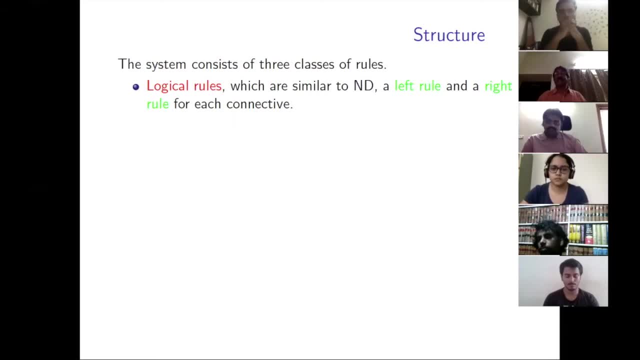 which is the part that is similar to natural deduction. In natural deduction, where you had an introduction rule and an elimination rule, here you have a left rule and a right rule Because you have sequence: there is a left-hand side and a right-hand side. 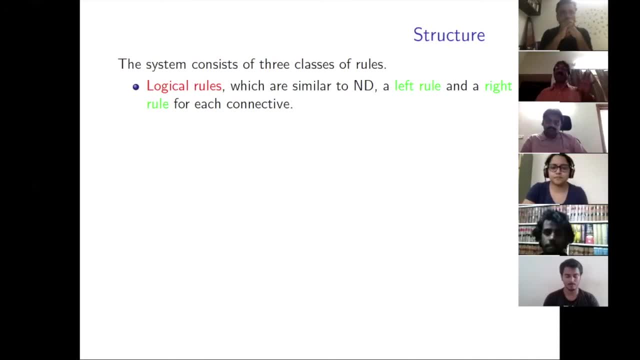 So you have rules that say: you know, I want to have this, So the Yeah, So you. So these rules are all. These rules are all reproduction rules in that sense Introducing on the left or introducing on the right, 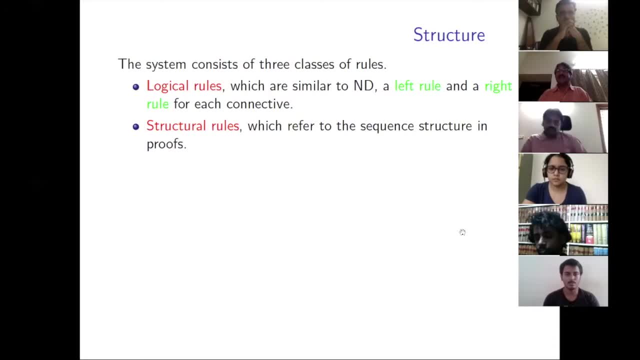 And then there are structural rules, which actually refer to the context or the sequence structure that you have. Uh see, remember that. uh, right at the beginning, I was saying that, uh, a proof is a sequence of formulas. 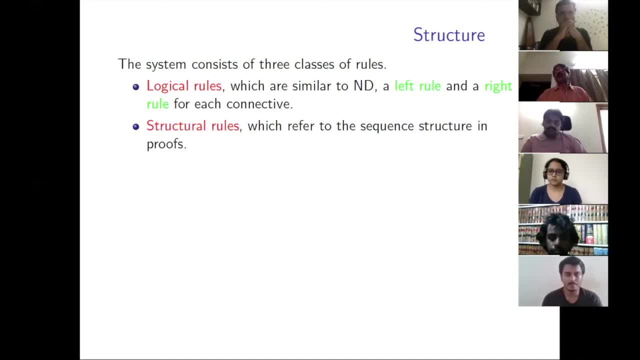 But if you really think about it, order matters. only for saying that I derived this earlier Right- And I use the inference rule modus ponens Right To derive beta. I should have derived alpha earlier. Alpha implies beta, But in terms of the logical content, 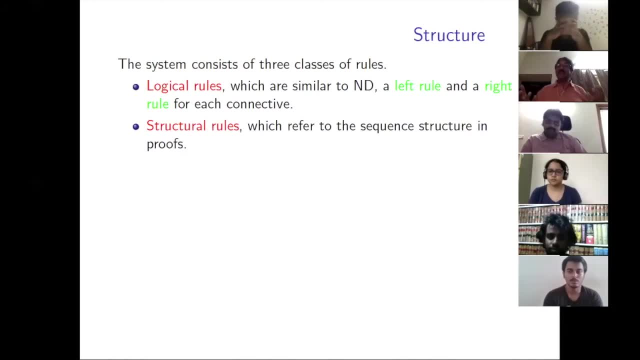 right, it hardly matters, Right? So the notion of time that you have, the sequencing that you have, how serious is it? Now, there are logics in which, uh, you know, uh, uh, supposing you are allowed to assume p or not, 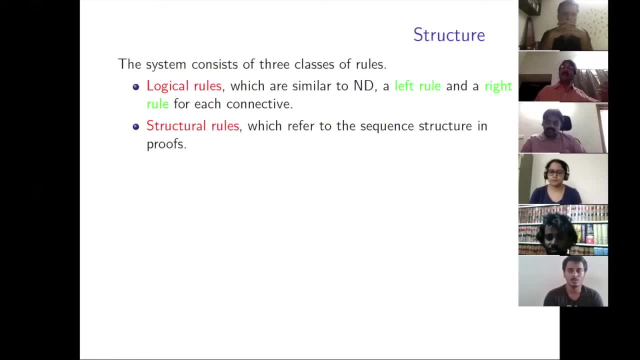 Right, Uh, whether you assume p first or negation, p first may matter because you know the further conclusions that you draw. Classical logic doesn't have this, but uh, Jensen was interested in having a very general idea around. 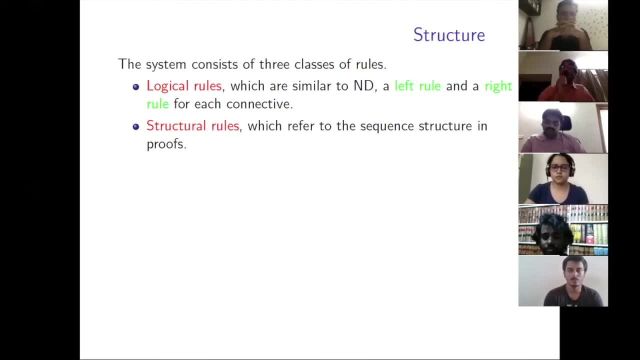 where, like I said, the context may actually matter, the order may matter. So structural rules are to explicate the dependence And then there are two core rules. So there are logical rules, structural rules and core rules. There are only two of them. 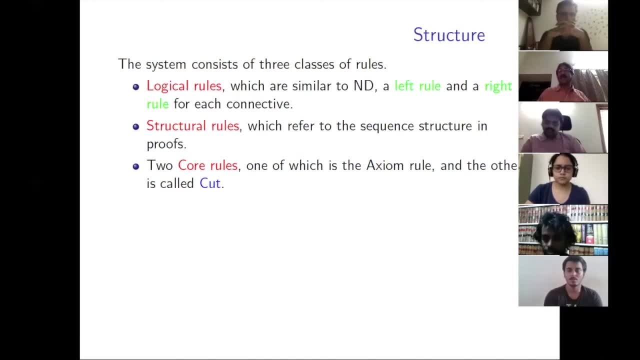 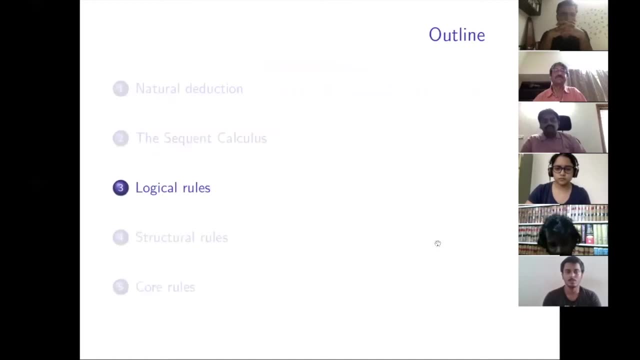 One is called the axiom rule, which is the axiom, and the other one is called the time rule. You will see that in a moment. So what are these rules? So first we'll take up the logical rules, because these are the familiar ones. 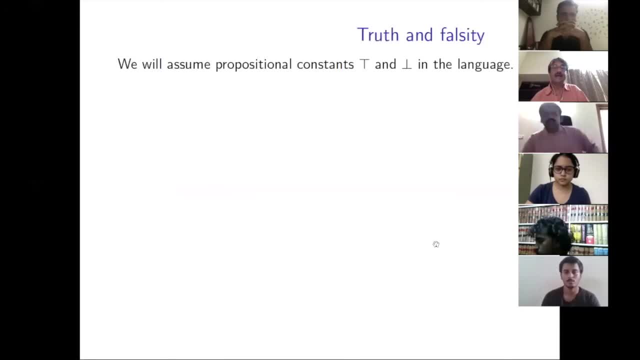 and the algebraic ones, And uh, so we'll assume that there are two propositional constants. Anyway, in natural deduction I already introduced a propositional constant, false, which is bottom side, But here we'll also use true. 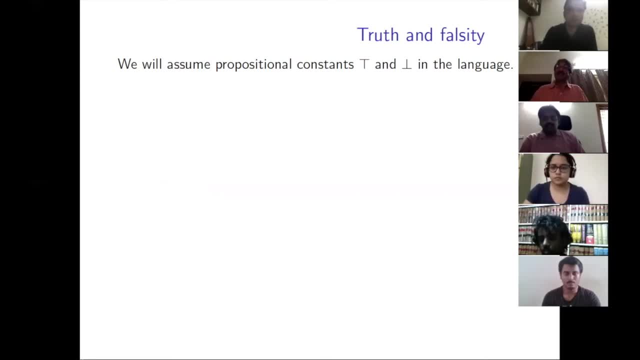 true and false. As I said for Jensen, now, everything there has to be dual. You can't have one without the other. So duality is there. So you have two constants, true and false. And uh, 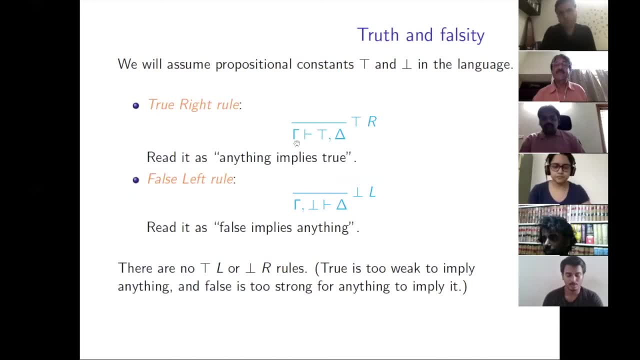 for true. there is a right rule. It says: well, gamma is any sequence of formulas. you have got Delta is any sequence of formulas. So this rule says that no assumption is needed. On the right-hand side, you can always put a true. 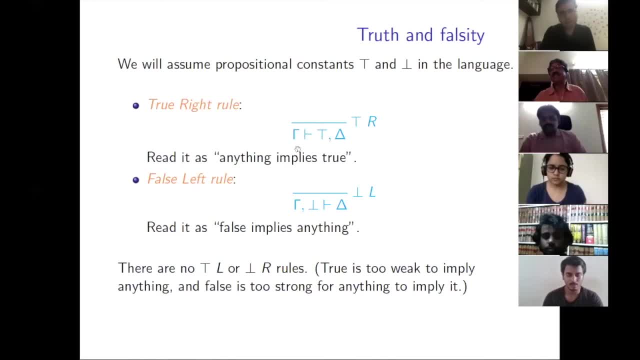 You can read it as anything implies true, Right. Whatever assumptions you make, I can always conclude true And in any context, Right, False, left rule. It says false implies anything Right. Whatever context you have got and whatever assumptions and conclusions. 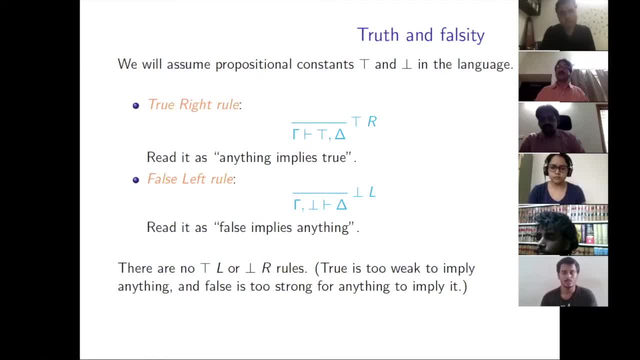 you can always throw in false on the left-hand side. False as an assumption is okay. So now you've got two constants in the language, two propositional constants. So you have to have right rule and left rule. Best thing is. 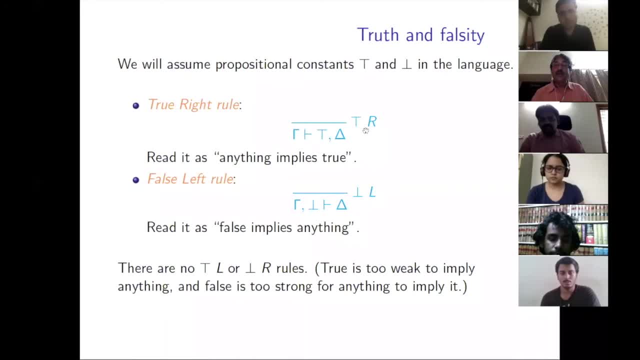 there are no uh left rule, first rule and second rule. So there are no uh left rule, first rule and second rule. So there are no uh left rule, left rule for top or 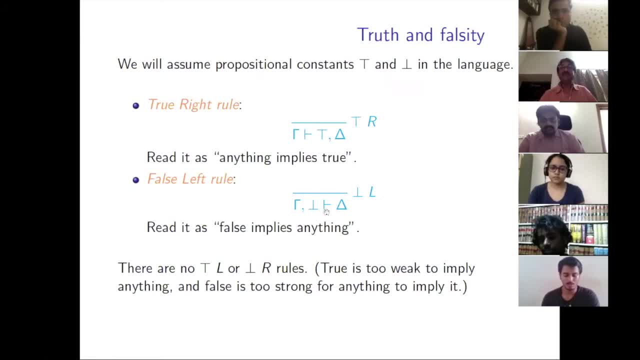 uh, right rule for bottom, Basically true. putting it on the left-hand side, well, true is too weak to imply anything Right And false is too strong for anything to imply anything You can't have. alpha implies false. 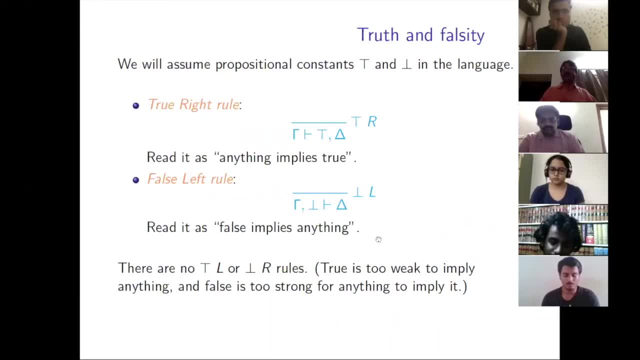 Right, So you have, and similarly you can't have. true implies anything except true Right. But then true you can always put on the left-hand side. So there are no rules for this. So these are not derivates. 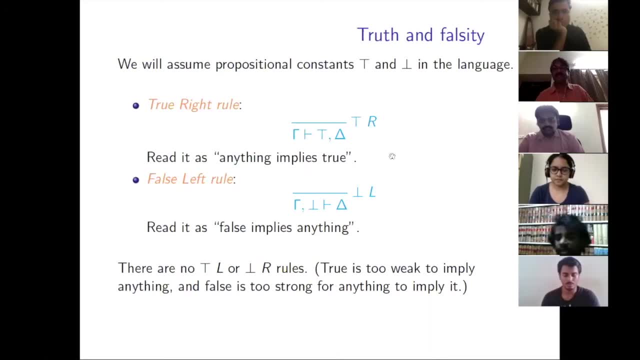 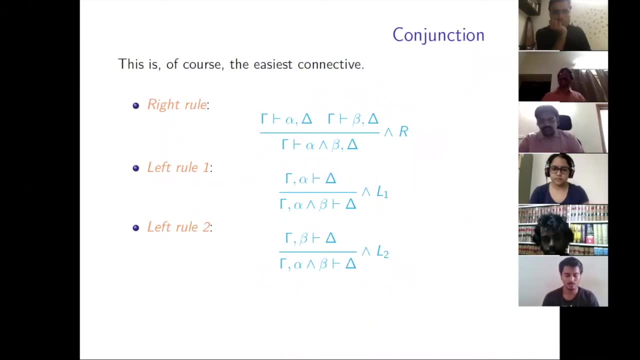 That's it. So this is the that's basically it. Oops, Then you have conjunction And that's the easiest connector. It's exactly what we have in the natural reduction system. The right rule for conjunction is if you have derived alpha on the right-hand side and beta on the right-hand side. 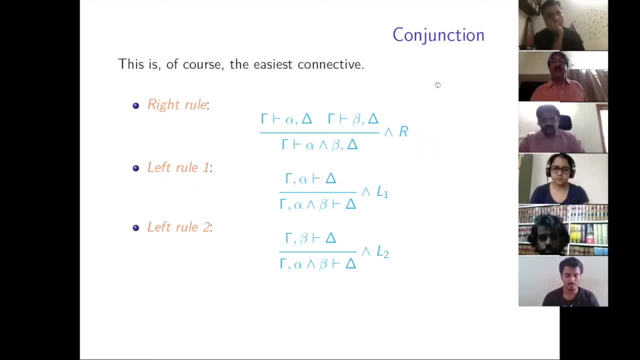 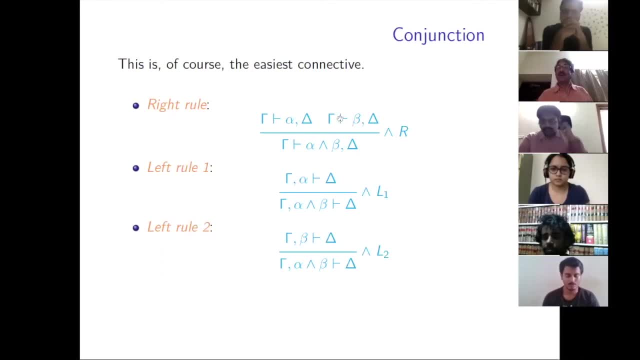 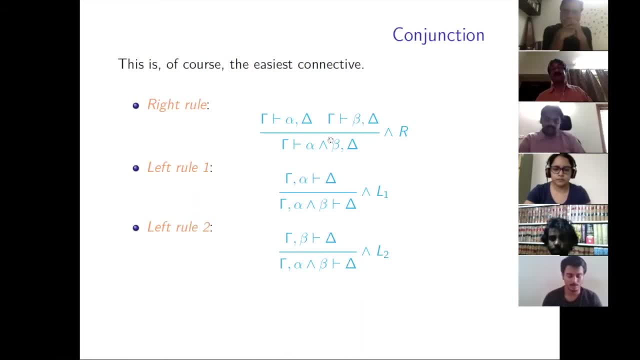 and, and, and and. Yeah, So you plug it in and check that this is actually true. So gamma implies alpha is valid, gamma implies beta is valid and gamma implies alpha and beta is valid in the presence of all the other disjunctions. 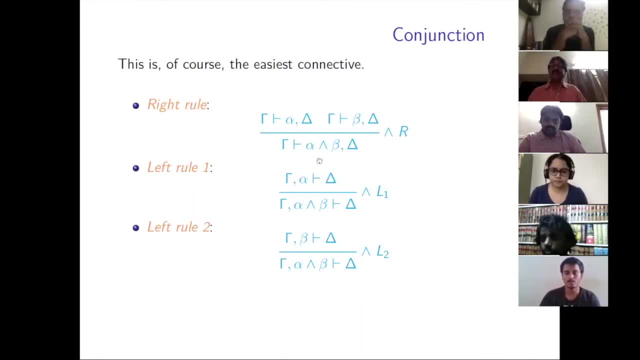 So the simplest way to make sure that you understand this is: consider a model that makes the gamma true, and if it makes this disjunction false, it will make all of these disjunctions false. in particular, it will make alpha and beta false. 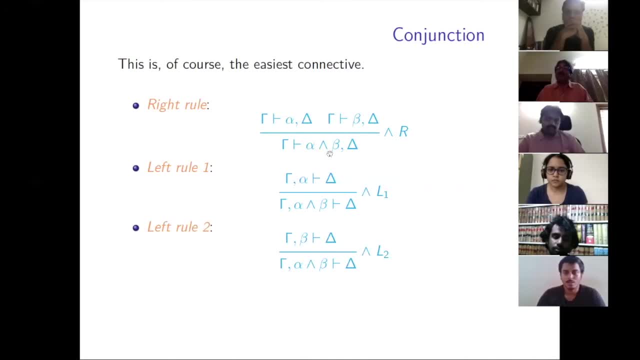 If that model makes alpha and beta false, it must make one of those things false. They say it makes alpha false, but then you're going to get a combination Because you know all of delta is false. So if gamma, if the model satisfies gamma and makes alpha true, it must make alpha true, essentially. 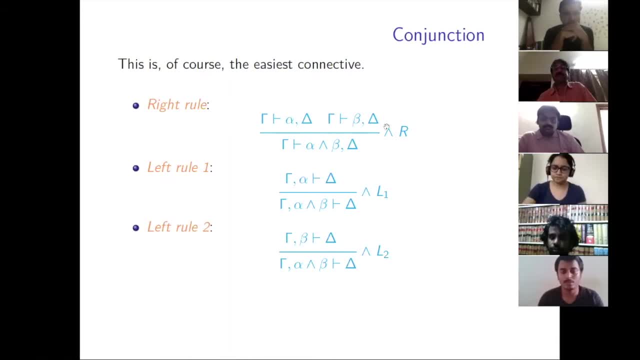 So yeah, so this is the right-hand side rule. And what about the left rule? It's exactly what you would expect. If you have assumed alpha, you can always assume alpha and beta. nothing will work Because the delta depends only on alpha and gamma. So adding an extra assumption doesn't hurt you, So you can add on the left side. so you have two rules. 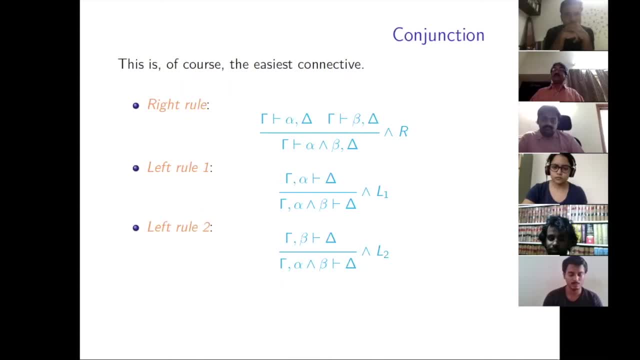 Now, so is the conjunction clear. So it also gives you an idea of how the sequential process proceeds. You have right rules and left rules. Yeah, that's the main idea, And uh, uh, uh, uh. So on the right-hand side you have to strengthen things. That's the point. 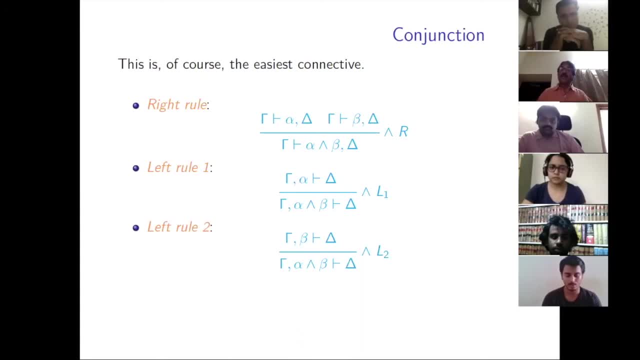 Right, On the left-hand side, it's assumptions, so you can weaken things. Assumptions can always be weakened. Conclusions can always be strengthened. This is disjunction. So now, what about disjunction Now? and this is the beauty of sequent calculus: you don't need to ask. 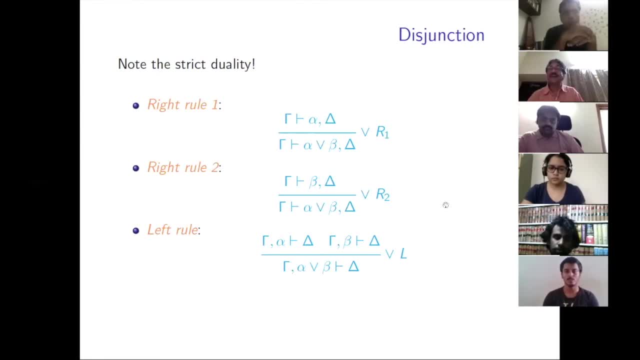 It's exactly dual. So, Uh uh, you don't have the kind of asymmetry that we have in natural disposition. Well, for conjunction, you had two left rules and one right rule. So for disjunction, you have two right rules and one left rule. 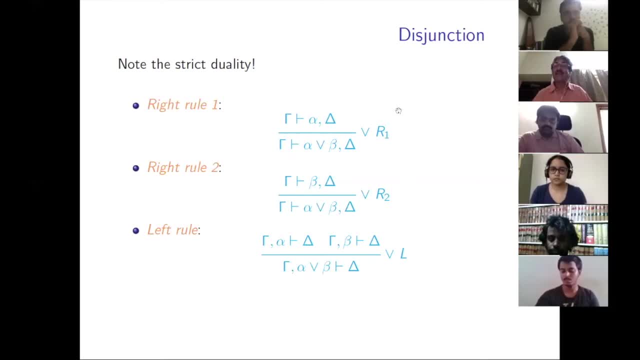 It has to be like this And uh for-. whatever you did for conjunction to the right becomes the same thing for disjunction to the left. So here, for instance, you have- if you have assume alpha and got something, if you assume beta and got something, it doesn't matter, throw in alpha or beta as the assumption. 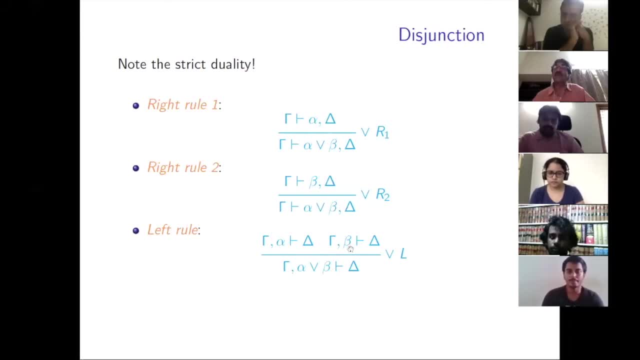 In particular, consider the case where beta is not alpha. This is the case analysis that we are talking about. Assuming alpha, you get something. Assuming negation alpha, you've got something. in all cases, That's a particular case. This is the general case. 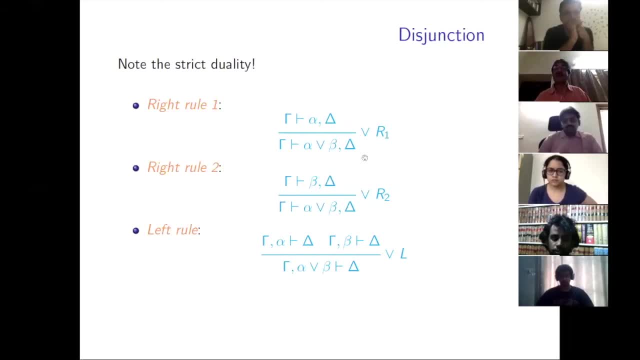 And here you're only weakening. You've derived alpha When you've concluded alpha, of course, you can always conclude alpha or beta. So this is the meaning of the assumption. Yeah, so is it clear? And negation is simply beautiful. There is no reduction of absurdum. there is nothing like getting a contradiction. all that is gone. 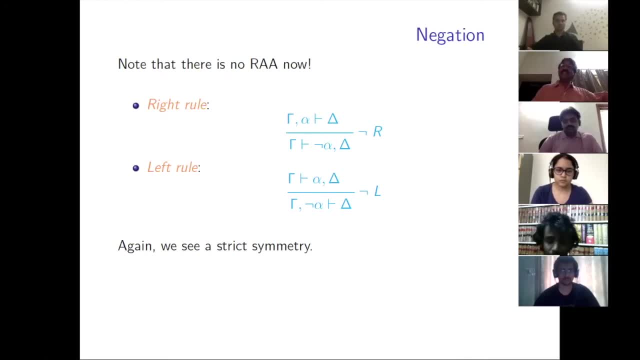 That is it. What is the right rule? It says: if you have assumed alpha and derived something, I can conclude negation, alpha or assuming alpha, I have derived delta, I can always derive either not alpha or delta. That's exactly what it says. And, symmetrically, if you have concluded alpha, 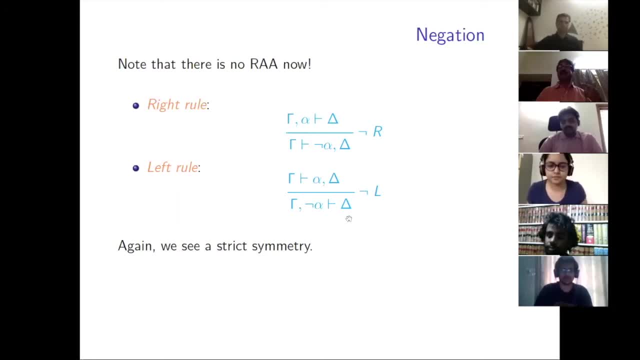 I can always make negation alpha as one of my assumptions, Right because we have already said either alpha holds or delta holds. So in the case where negation alpha holds, delta must hold. That's the meaning of negation. So it simply moves left and right. 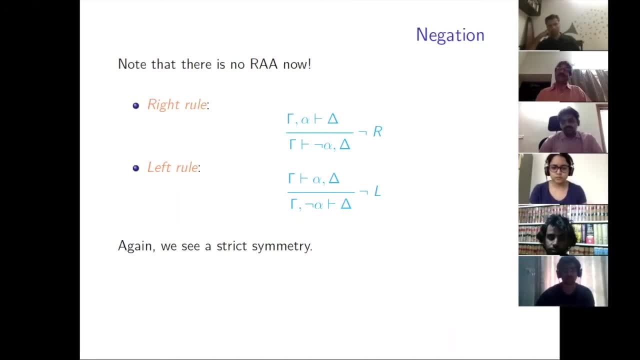 That's all Like we did before. So it's a strict symmetry and that's very important. Is it clear? Again, check the soundness. Assume this is you know, gamma union alpha gives delta as a consequence. We want to show that not alpha or delta is a consequence of gamma. 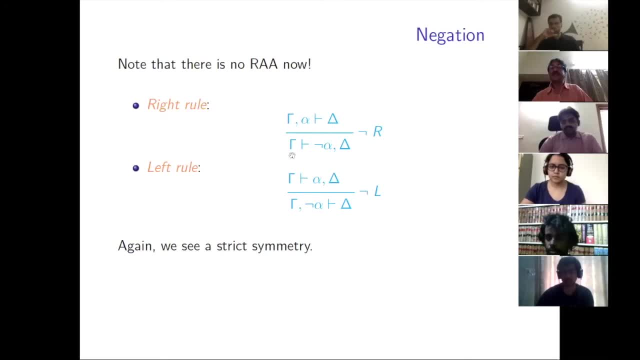 How do you show that? Take any model, Assume that it makes all of gamma true. Then we want to show that it either makes alpha false or delta true. Okay, Suppose the model makes alpha false, you have true. Otherwise, the model makes alpha true. 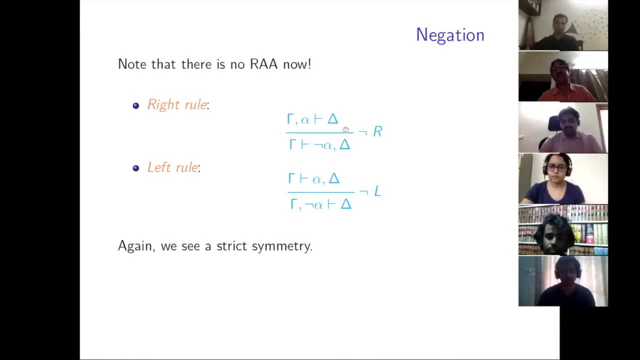 It makes all of gamma true and alpha true. Therefore, it makes all of gamma true. So these are all, like you know, fairly natural things to But beauty now is the symmetry that you can make yourself, The structure in the, And what about implication? 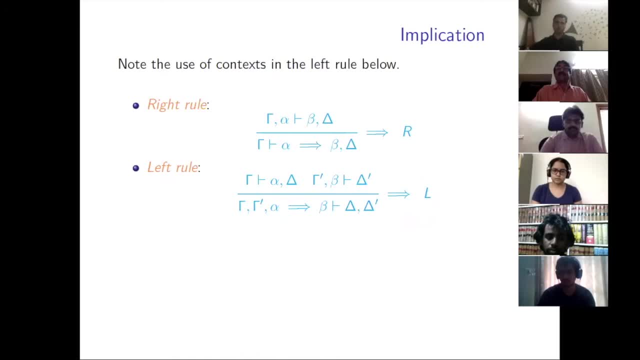 And this is where the use of context comes in. The right rule for implication is what we have talked about as one part of the reduction theorem. The difficult part of the reduction theorem that we proved in the Hilbert calculus is the right rule here. 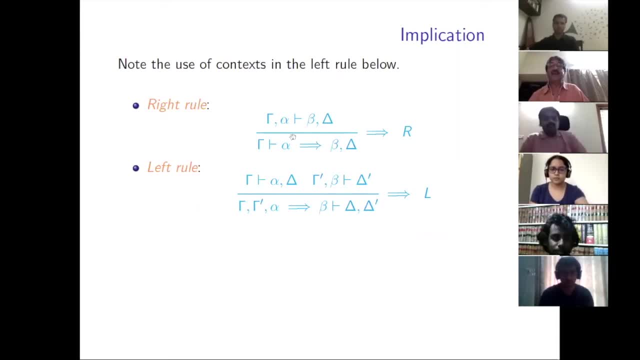 The difficult part of the reduction theorem that we proved in the Hilbert calculus is the right rule here. The difficult part of the reduction theorem that we proved in the Hilbert calculus is the right rule here. That is, if gamma union alpha gives you beta, then gamma gives alpha implies beta. 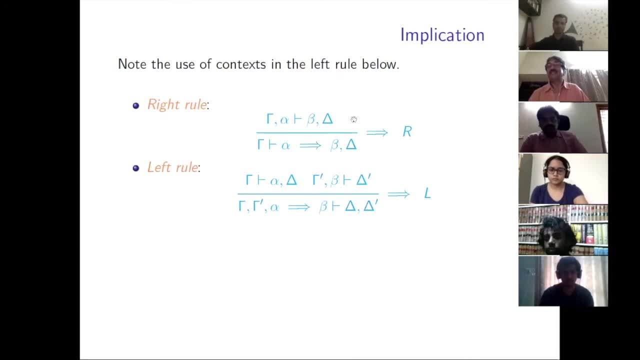 Of course, you are doing it in the presence of other disjuncts. Is the idea clear? Again, this is sound, right. I mean, this is in fact, as I said, And in terms of consequence, it's very easy to see. 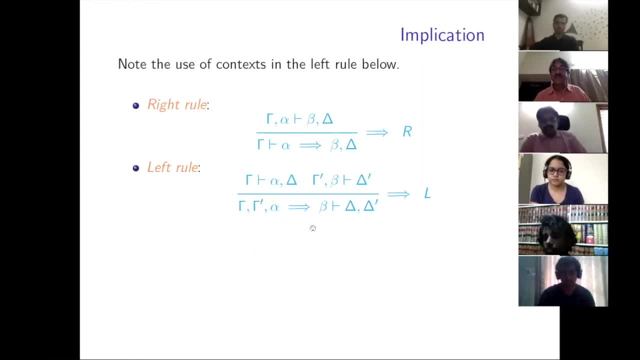 But what about? how do you bring alpha- implies beta- to the right? But what about how do you bring alpha- implies beta- to the right? And the rule is a little more complicated. It says: assuming gamma, I have derived alpha And in another context, assuming beta, I have got beta. 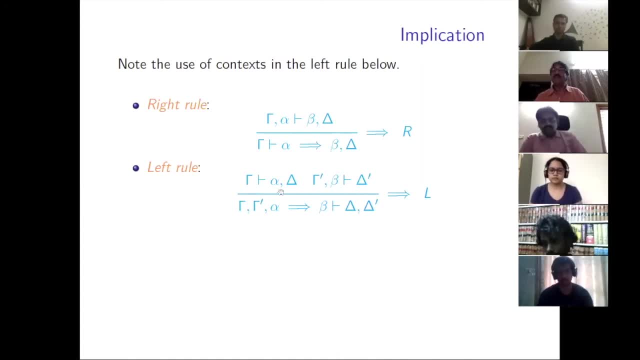 Then I can combine the contexts. Note that these two proofs see. unlike the earlier proofs, Here it's the same gamma For disjunction and conjunction. I must use the same context, The same set of assumptions. I have derived alpha and beta. 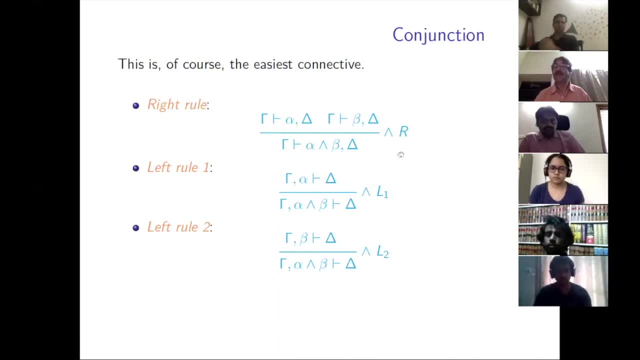 It's very important- You can't change the gamma, Whereas- and this is what natural reduction is telling you. As far as implication is concerned, if you are going to make implication part of your assumption, then you can also think of things from different contexts, as long as you find. 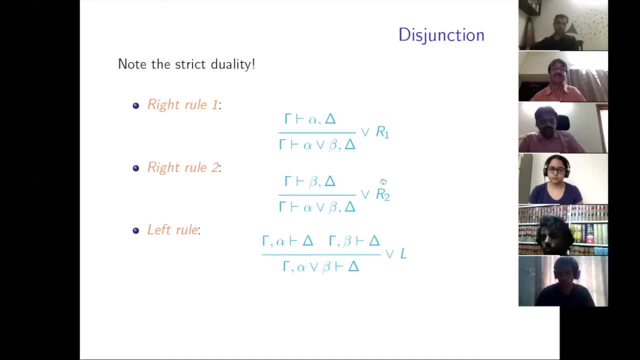 So this turns out to be extremely easy. So once again, to see the soundness, assume that these are. assume consequence here. Consider a model that makes gamma gamma find true and alpha implies beta true. You want to show that it makes either delta true or alpha find true. 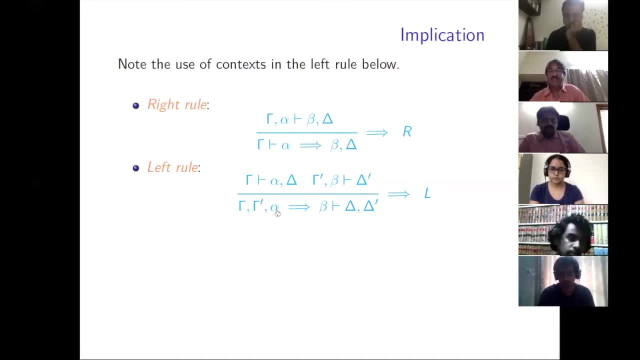 Well, we know that the model makes alpha implies beta. true. So in that model either alpha doesn't hold or beta holds. Suppose beta holds. this tells you. well, this model makes all of this true. Therefore it makes gamma find true. 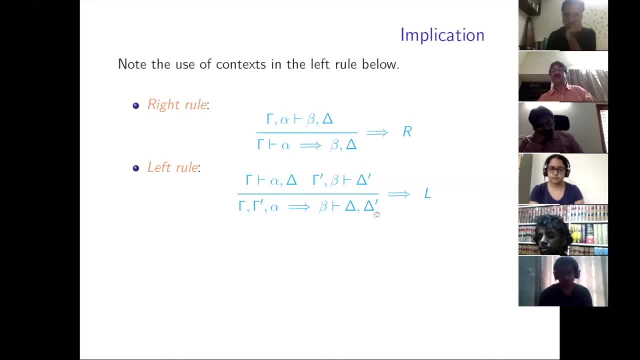 It makes beta true. Therefore it makes delta find true. If it doesn't make alpha true, yeah. So this is the two cases: It makes alpha true, it must make alpha true And otherwise, yeah. So in this case you notice that it satisfies all of gamma. 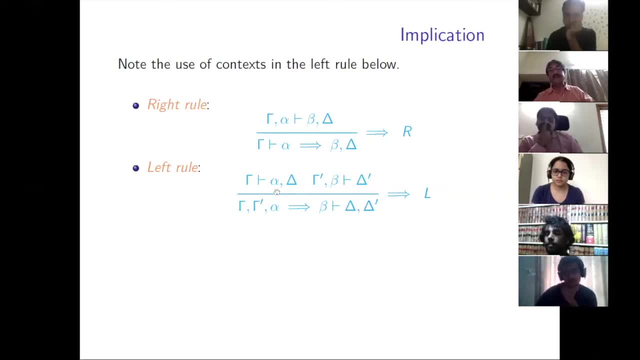 So it must satisfy one of the discharges. So either it makes alpha true or delta true. If it makes alpha true, we are happy. So it's a fairly, And so this allows us to do precisely the sort of things that we were talking about earlier in natural deduction. 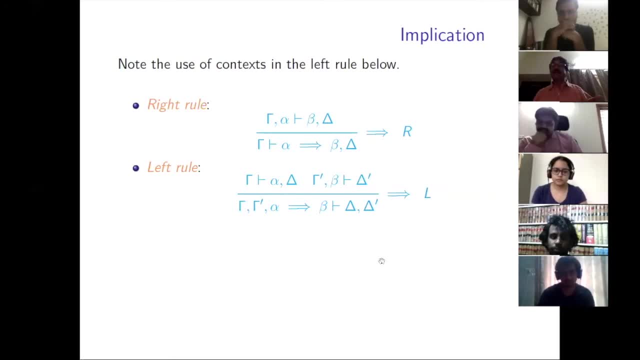 But that made different. The main difference is that you know in natural deduction there is a scoping rule which nests assumptions And that nesting is gone. So you can simply. So. if you recall, I pointed out that in natural deduction, if you keep making assumptions when you discharge them, you can only discharge the innermost. 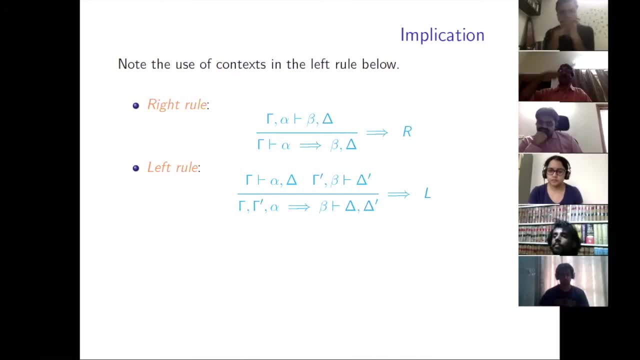 And then the next outer one, the next outer one, So and that creates, you know, problems in, Like I said, it's okay for you know, I think it works reasonably well for human beings. But if you want to in general talk about existence of 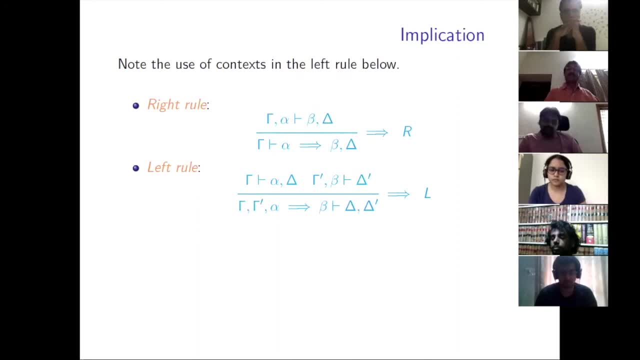 It's not easy And this provides a And at the point. this also shows you. I think it's very important to realize that there are lots and lots of proof principles around right. If you just start with the notion of semantic consequence, I mean, these are all, all these rules, preserves. 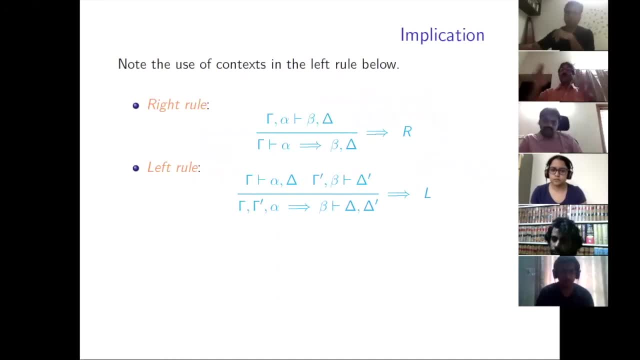 So there is a choice, right? So what is true out there? you know there are many arguments, But if you want to use a finite computational deductive apparatus, you have to make certain design choices About what you have available on the house. 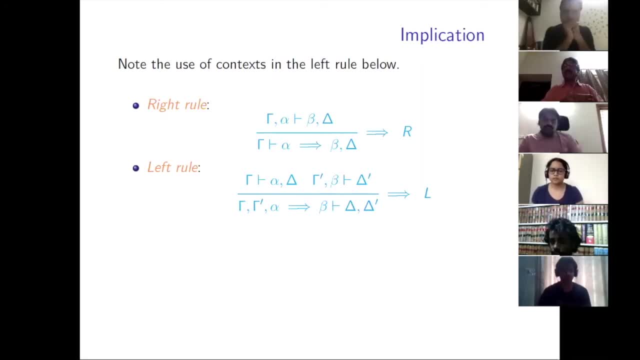 And that's why I said the connection with the programming language theory is very strong. The constructs that you use and how you reason, you know, compose these constructs is very important. That's what Jensen had very nicely said. So these are the logical rules. 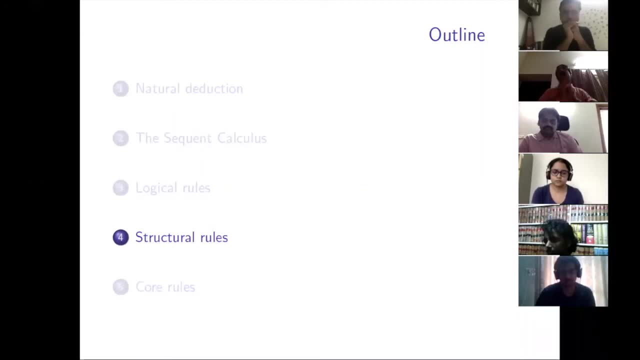 For the propositional constants, true and false, we had right under there. That proves Then, for negation, Conjunction, Disjunction, Multiplication, For all of them we have got. So now we go to the structural rules. 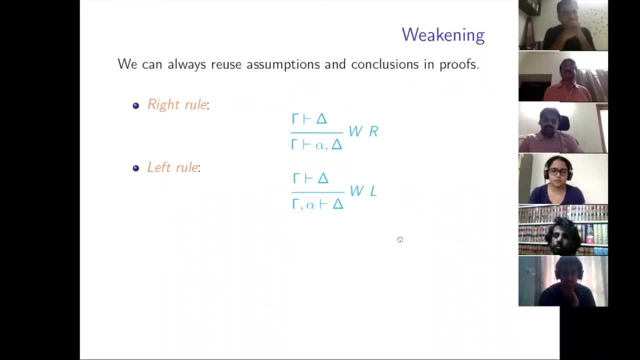 What are the structural rules? The first set of the first is weaken. It says that, yeah, you can always, you know, weaken your assumptions, Yeah, And strengthen your conclusions. If you have already derived delta from gamma, then you can always write alpha or delta. 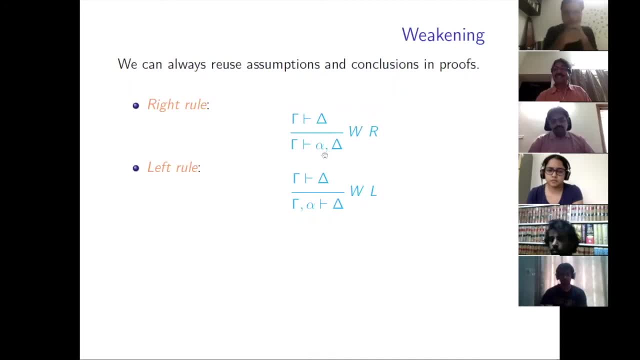 Right, No problem. This just says that comma on the right hand side behaves as disjunction, Right? Remember there is no comma in the logic, The commas that are there in sequence. So this actually tells you that, Because if you look at the right hand side, 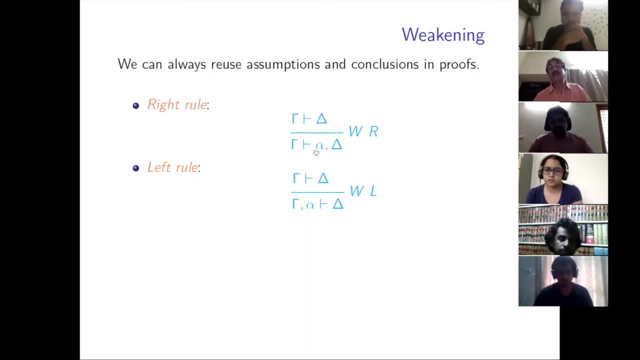 The right rule for disjunction that will use alpha or beta. You have alpha above and alpha above, Whereas this says: I can always add an element to this. So this is the formal meaning of saying on the right hand side, whatever you've got behaves like disjunction. 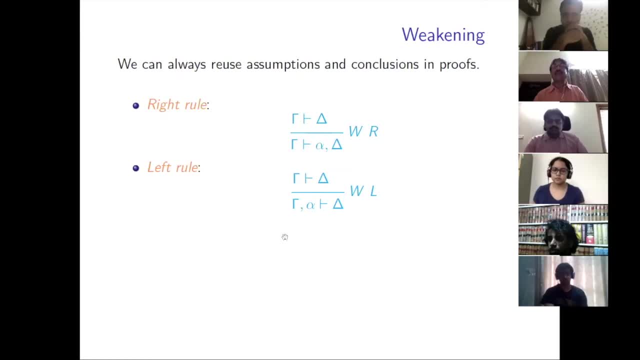 And this is the one that says that whatever you've got on the left hand side behaves like disjunction Right. So I hope that is clear. Then this is weak, This is contraction, And this is to do with the fact that, even though we write sequences, we don't really use sequences. 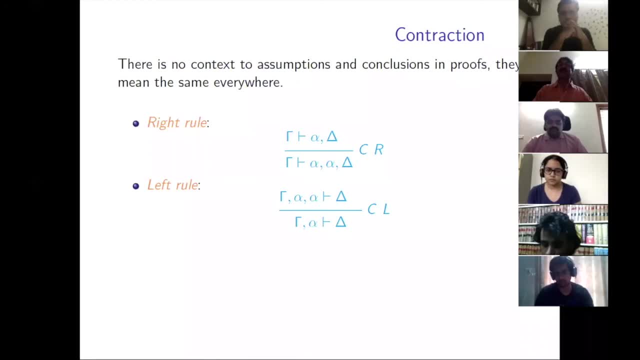 Right, In the sense that alpha or alpha is the same as alpha And alpha is the same as alpha, In particular, when I am writing assumptions, how many ever cop? you can reuse assumptions as many as you want. So this is what I am trying to do. 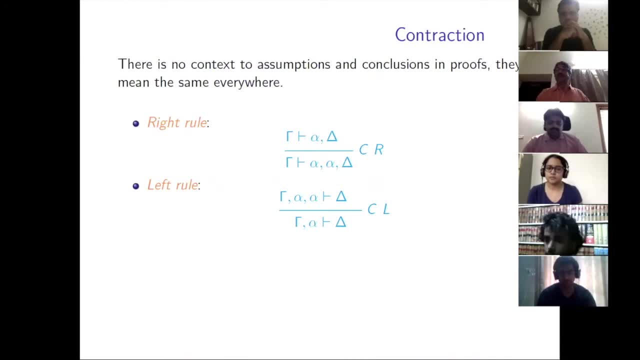 Right, You can reuse conclusions as much as you like. You can reuse conclusions as much as you like. They are for free, Right. And so there is no context dependence to assumptions and conclusions and proofs. They mean the same everywhere. 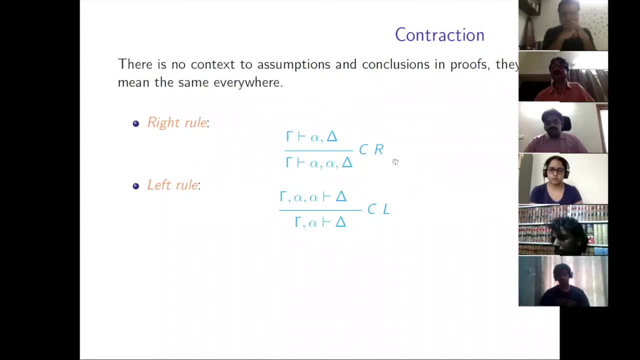 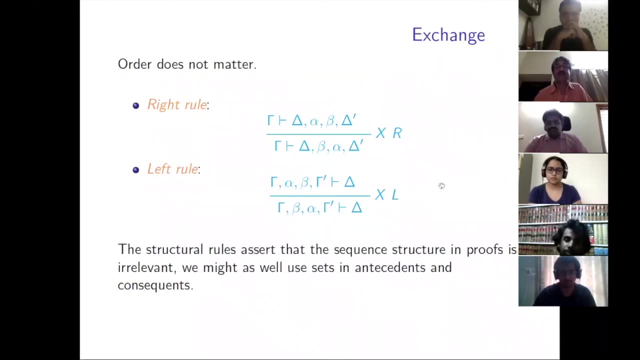 This is everywhere And for Genshin. you know these are things not to be taken for granted And, as you can see, there are logics where you don't need them. And one more: It says order doesn't matter. 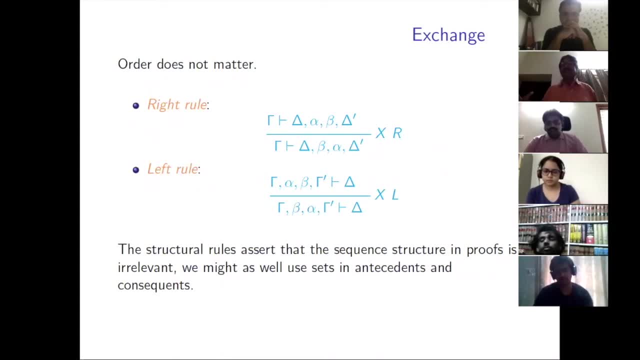 Right, Even though we write sequences. So basically, what we are saying is that these are really sets Right. They are sets because the order doesn't matter, Repetition doesn't matter. So the main order, dependence of applying the rules in a particular way, all that is gone. 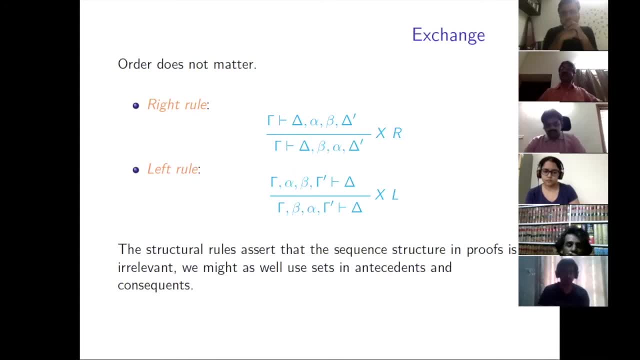 It's just sequence And we write sequence upon sequence, Using whatever order it is. So this you know, Sir. Yeah, No, okay, sir, I have a question in the left room. It's all right. 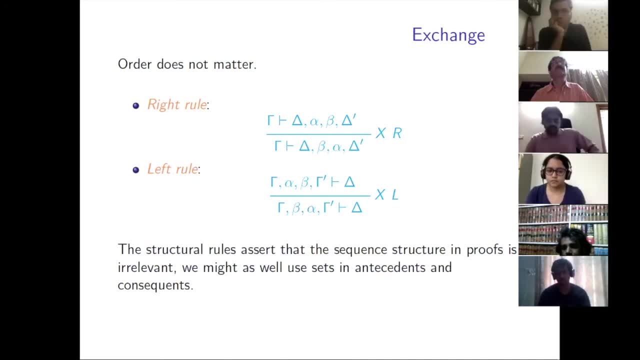 Yeah, Is it okay, Sir? my question is that this delta, delta, prime, they are also sequence of formulas. Yeah, yeah, They are all sequences, Yeah. So, sir, Why not just write, Just write alpha comma, beta, then beta comma, alpha. 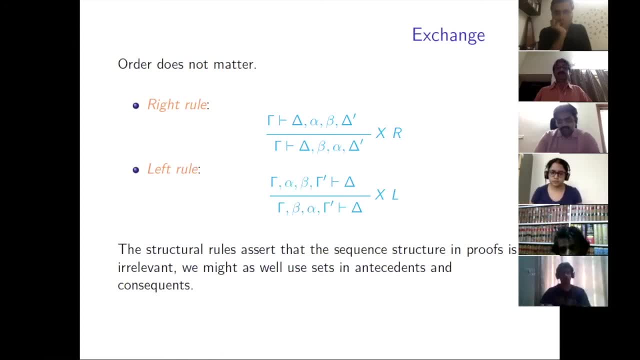 Why do we have to add delta and delta prime? No, no, What we are saying is that you know you can do the swap anywhere in the middle. is what it says, Right, By putting delta and delta prime on both sides. I am saying that you can do the swap anywhere. 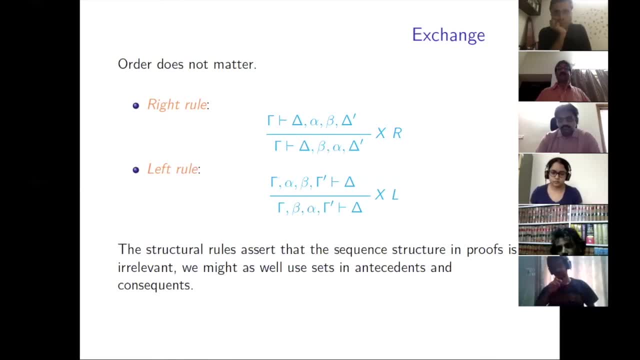 within the sequence Yeah, Okay, okay, You can do the swap here on the right hand side. You can do the swap on the left hand side. Otherwise it might be that you can. you are allowed to swap only at the right most. 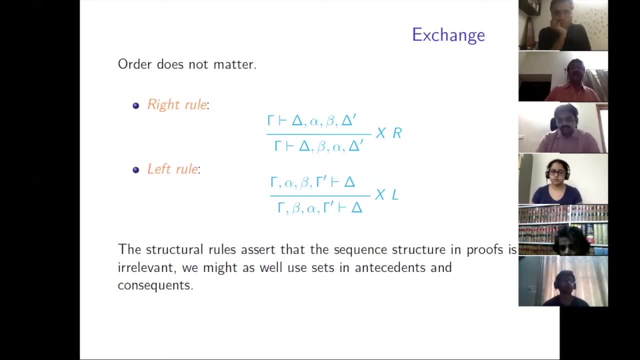 or only at the left most end? Yeah, And of course you can have a again. you have a choice of many possible rules. Right, You can always swap at one end and keep pushing all the way. Right, You can do that. 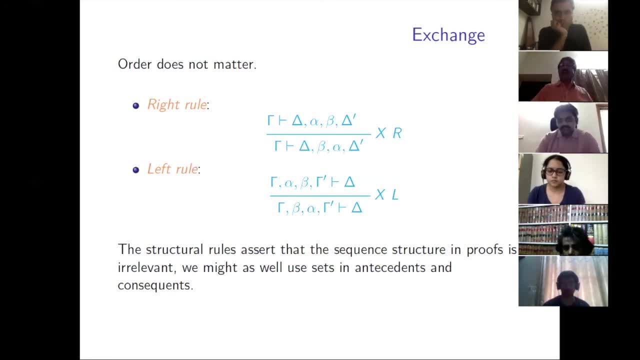 But you know that will blow up your rules And also it may create all kinds of complications. Yes, Thank you. Yeah, So the structural rules assert that the sequence structure in groups is irrelevant. We might as well use sets in as antecedents and consequences. 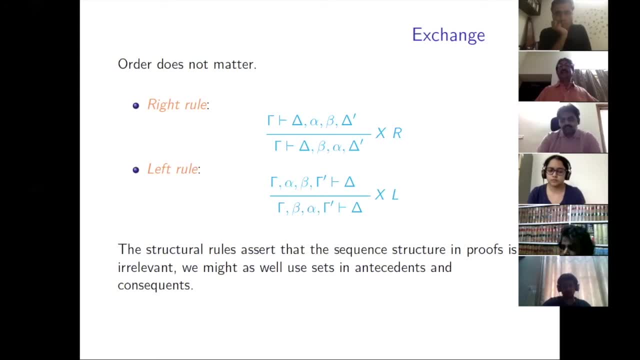 By the way, I never mentioned the term that gamma on the left hand side is usually called antecedent and delta on the right hand side is called antecedent. Yeah, In fact Benson called them sequence, But Kleene was the one who called it a sequence because you know, the German term is too. 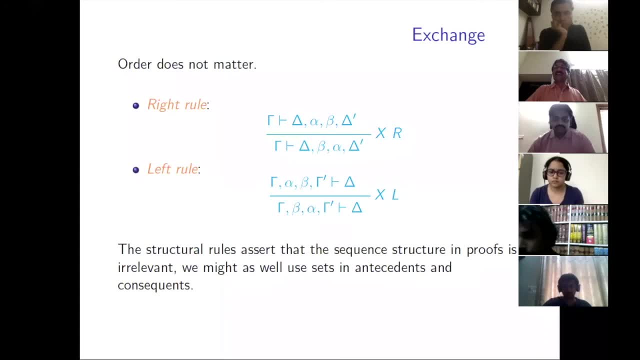 close to the word sequence in English, So sequent is for him. If you read Kleene's book Introduction to Metamorphosis and Kleene actually says that Kleene is some complicated reason for you know you take this part from antecedent. 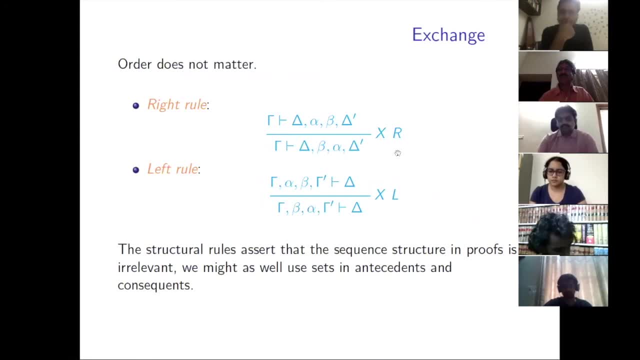 this part from consequent. But Kleene is worth reading. I mean, it's for me. I would say. one of the books that made a major impact on me was In Care. Parallel Introduction to Metamorphosis. Okay, 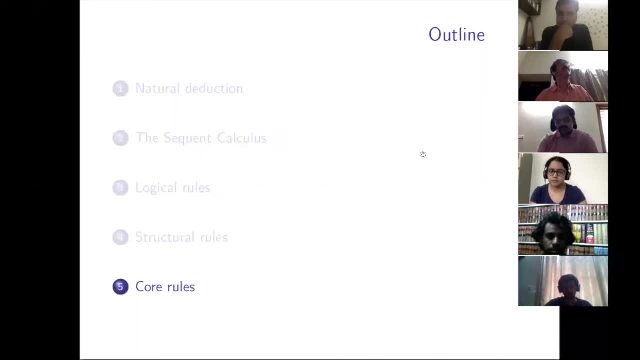 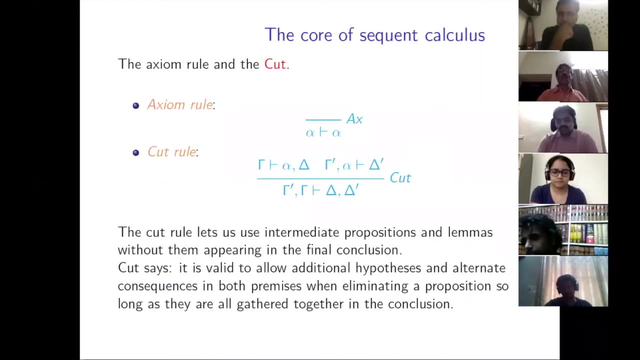 So we are pretty much done with the description of the system. So we have looked at the logical rules, We have looked at the structural rules, And then I said there are two core rules. One is the axiom rule And this is alpha from alpha. 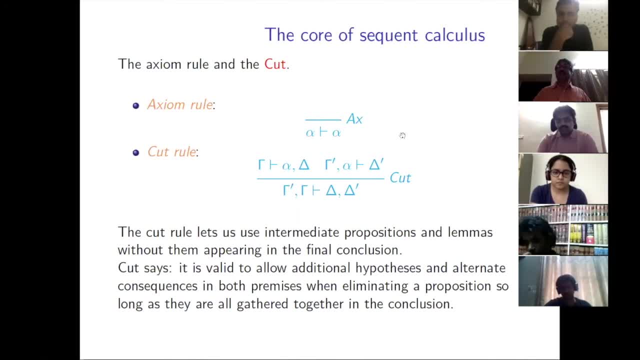 Of course that's axiom. And then you have the cut rule. What is that? This is the only really complicated rule. And yeah, and it's something to see what it says. What does it say If I have assumed alpha and proved something and later I have established alpha, think? 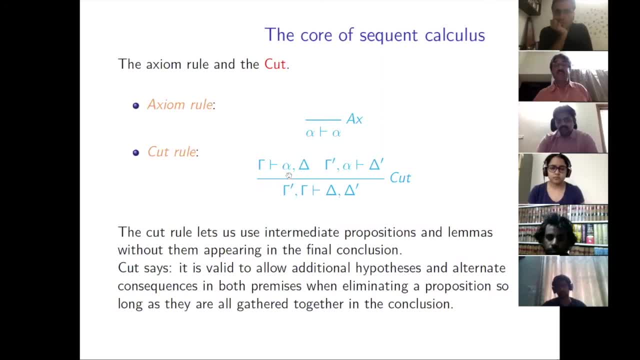 of it as a lemma. If you have established the lemma, you can use it and then prove something. then you can get rid of the lemma. You make a claim, settle the claim and get rid of that. That's what it says. 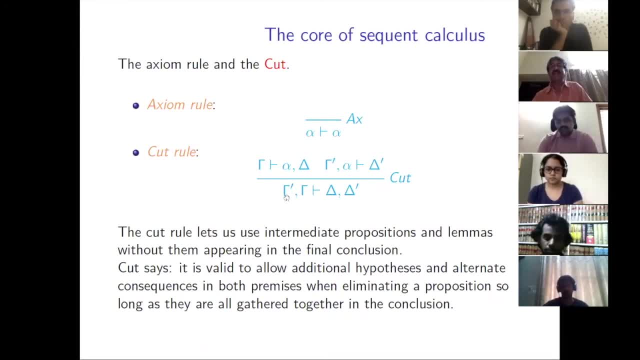 So it lets us use intermediate propositions and lemmas without them appearing in the final conclusion. In one context I have derived alpha. In another context I have assumed alpha and proved something Combined the contexts. It says it's valid to allow additional hypothesis and alternate consequences in both the premises. 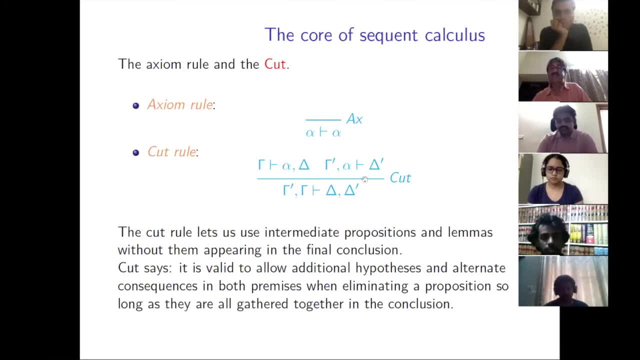 that you've got here when you eliminate this proposition alpha. Okay, As long as you gather together in the conclusion carefully. That's what it says, And this is very nice, because in sequence calculus, like I said, you do things in different contexts and put them together. 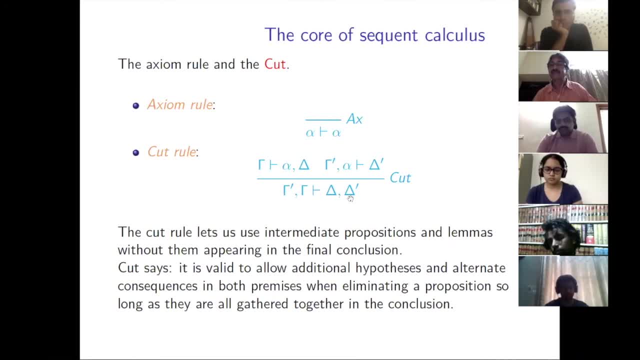 You have to make sure that you carry. As long as you carry the context down, clearly it's okay. So this alpha has simply disappeared from the conclusion And so these are intermediate solutions And again, in terms of soundness, you can see that this is true. 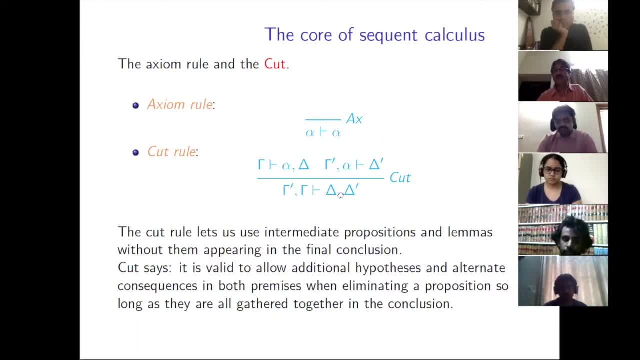 Why? Well, consider a model that makes all of this true. We want to make either delta or delta prime is true. Well, if this model makes all of this true, That model either makes alpha true or it doesn't. Suppose it makes alpha true, since it satisfies it. 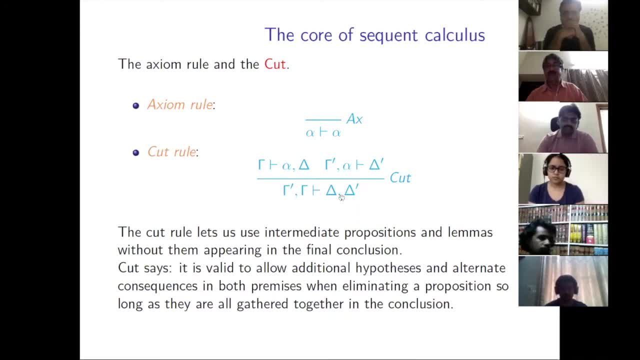 Makes all of gamma prime true and alpha true. It must make delta prime true. Therefore it makes this assumption. Okay, Well, suppose it doesn't make alpha true. Well, it made gamma true, Therefore it must make alpha or delta. 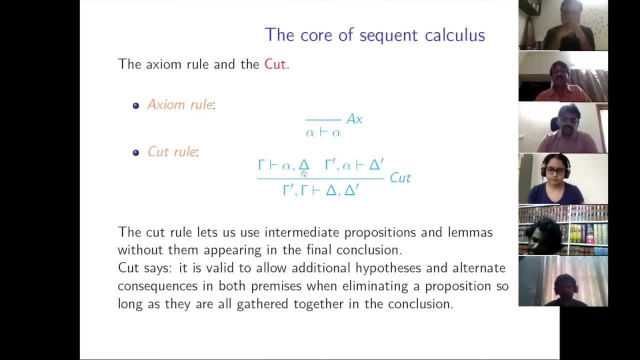 Well, we have already said that the model makes alpha false. Therefore it must make delta true. Therefore it makes delta true. But that's verification. The intuition behind cut is really this idea that something like what you do in natural deduction 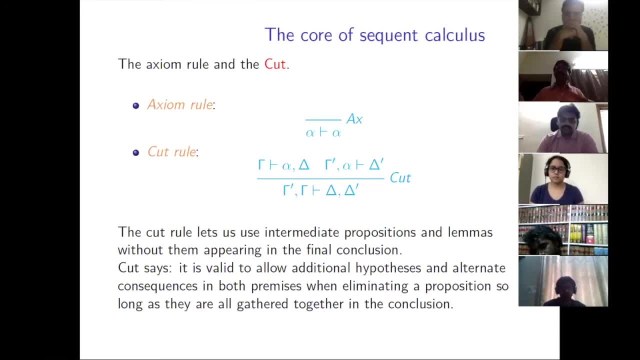 You make assumption, But it's not that you discharge them by doing implication and worrying about slope and so on. No, You make an assumption. That's some proof somewhere. There is another proof somewhere where you have actually established and there are certain assumptions. 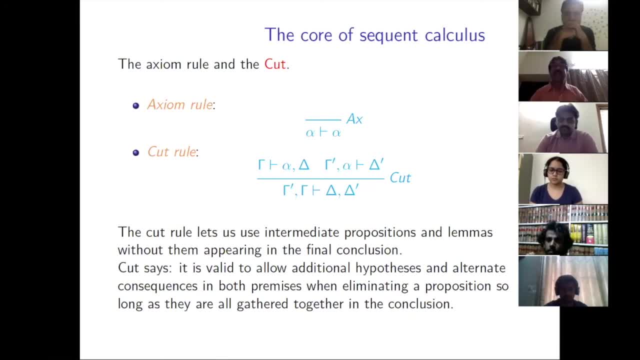 Combined assumptions and conclusions And here you have cut out alpha from these two groups. That's why it's called cut, And this is a very important And it's actually cut that lets you get rid of all the problematic ones. Remember, there is, you know, there is- no reductio ad absurdum. 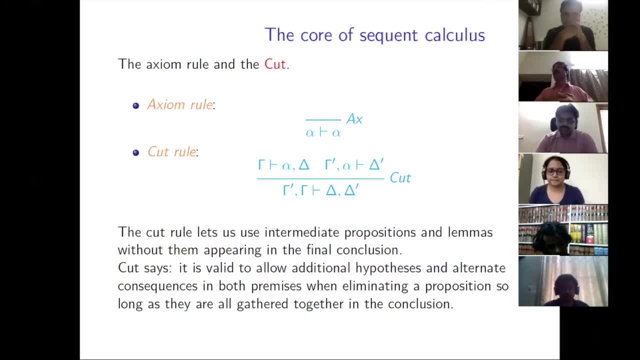 None of these things, Right. And I told you that the was bothered by the fact that, in natural deduction, negation appears in all these funny things Right. And here it's. So what happened? And that's you know. you see that when you actually do the, 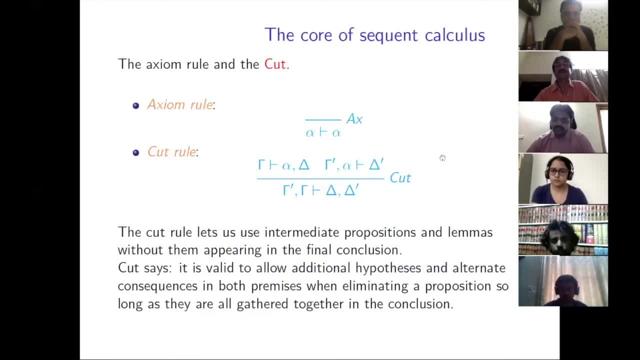 Cut is something that's, But yeah. So if you work in intuitionistic logic, for instance, in intuitionistic logic, you cannot assert alpha or The whole point of intuitionistic logic is that reductio ad absurdum is not a model. 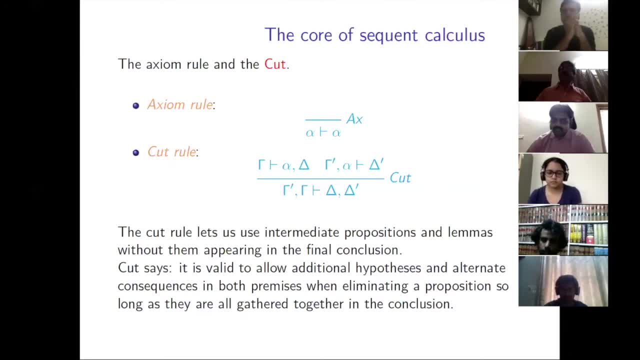 Only in a particular form, And so you have to be very careful When you can. In particular, you know, in intuitionistic logic you cannot have contradictions Right, So from contradiction anything But alpha or not alpha is not, And this is something that 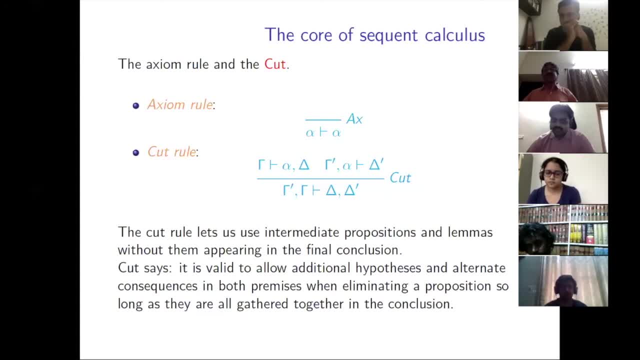 And especially for you know, there are a lot of parts of mathematics where you assert the existence of objects by saying that, suppose the object didn't exist, Something happened, Contradiction. Therefore it must exist, And you know. 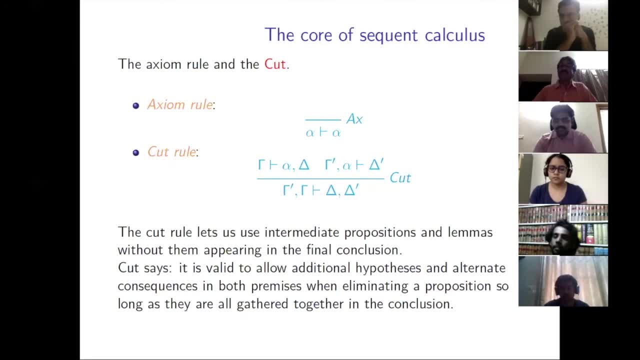 So how do you show the existence of an object? by not producing the object, but by getting a contradiction from Anyway. So sequence calculus is very, very neat, as you have seen. I hope you agree with me that it's a. Can I ask a question? Yeah, Please Yeah. 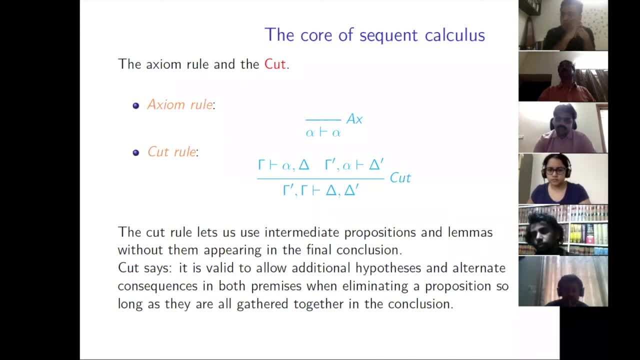 But modus ponens is expressed in terms of implication And we have this implication- introduction and elimination rules- in sequent calculus anyway, I mean the left rule and the right rule. So how are these to be seen as reflections of each other? 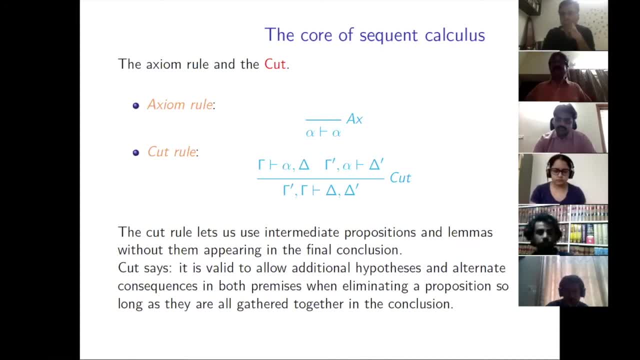 OK, so I mean, of course, the sense of completeness, right. Everything variable in one is variable in the other, But the proofs look completely different, Like in the natural reduction system and the Hilbert system, you know, after all, implication elimination. 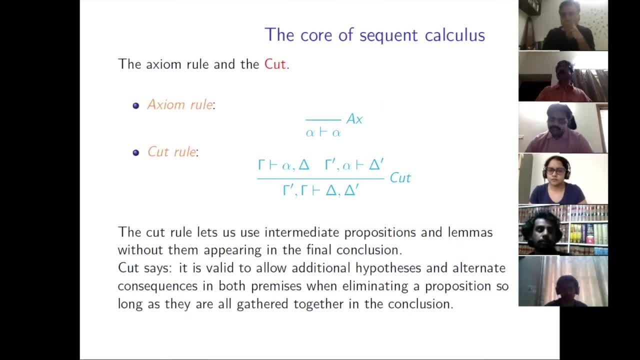 is modus ponens right, That's what you're asking, But how is implication introduced? Implication is introduced in natural reduction system By making an assumption alpha, deriving beta and then discharging the assumption to write. alpha implies 2.. 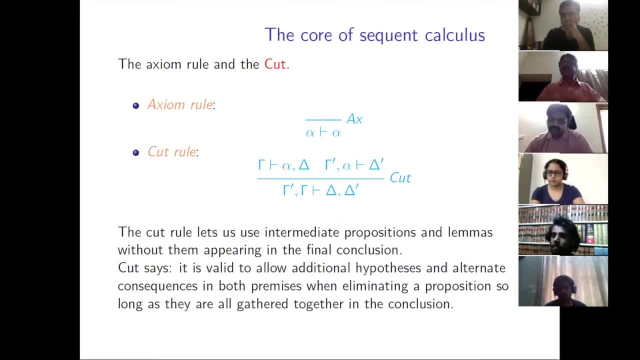 That's how you do the introduction right Now cut doesn't have any of that. The main point about discharging assumptions, as I said, by implication, is that you carry the context into your formula. That is why the nesting of contexts in natural reduction. 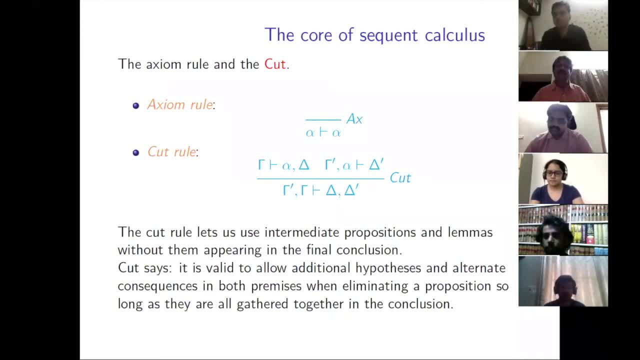 is a complicated process. None of that. In cut, you just have to do it. You just have these, as I said, these different contexts, And here you do it entirely through conjunctions and disjunctions. That's the difference. 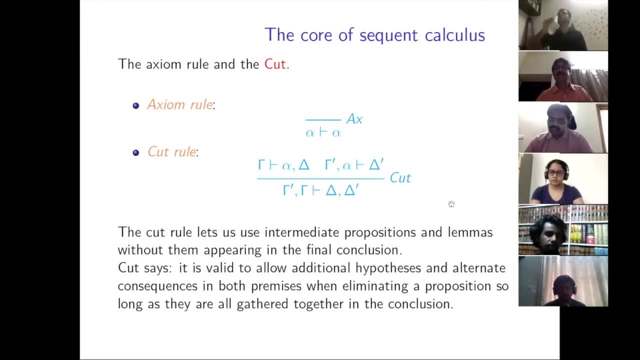 OK, Sir, Yeah, Yes, sir, I was just thinking like this cut rule, there is some similarity with the transitivity of consequence relations. There is some similarity with the disjunctions which we prove, like reflexivity, monotonicity and transitivity. 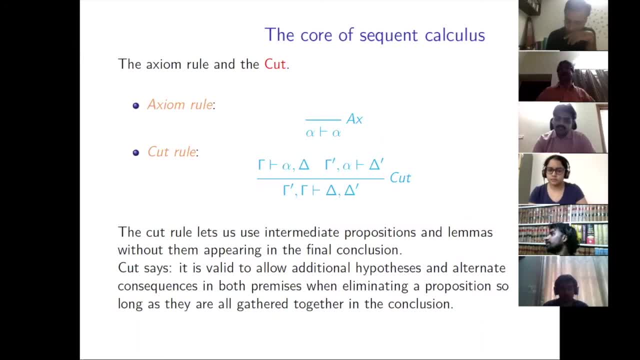 Yeah, So that each conjugate, Yeah, I mean that is the soundness of this rule. The soundness of this rule is basically from that: Yeah, But as I said, the semantic consequence relation has all kinds of properties To get them into proofs in some particular. 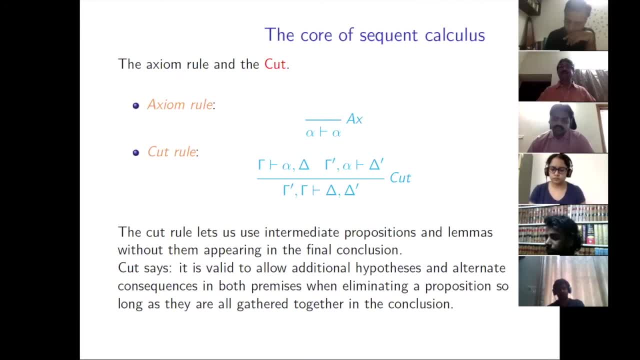 and remember those are with infinite sets. Here you have only finite sets. Yeah, Yes, Yes, Yes. The main point is that you are trying to capture something infinitely like the semantic consequence relation and its properties using something finite. 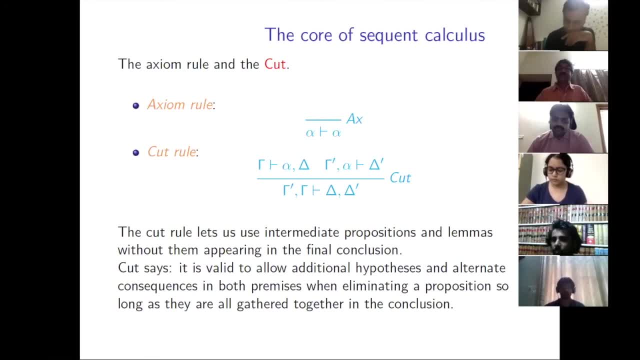 Right Proofs are finite objects, And so we want a strong enough rule that captures one of them, And cut is one of those things that makes a choice which turns, And, by the way, all I'm saying is also related to mechanization. 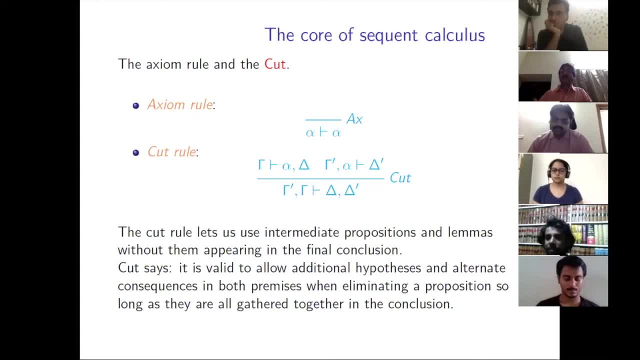 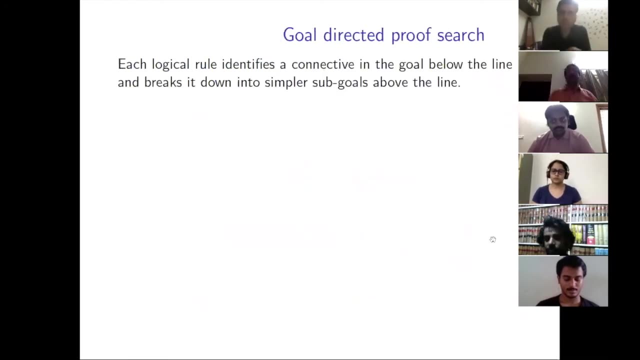 Right. We are moving away from the way human beings do proofs to a completely structural way of doing proofs, And that also means about mechanizing. So this is all about goal-directed search, Each logical rules identify a connective in the line and breaks it down into. 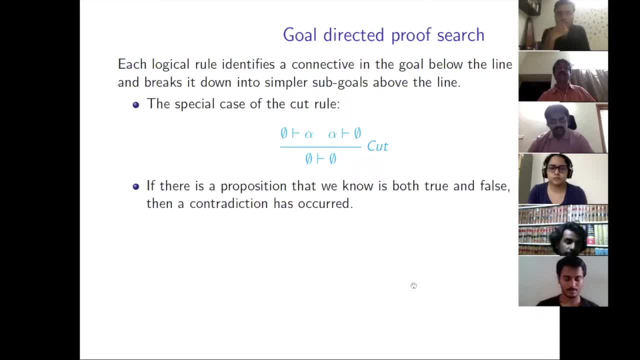 about the line. This is very similar to, And look at the special case of the. What does it say? Suppose I mean I have used the empty set, I should write empty sequence, Because by now we So from the empty assumptions you have derived alpha. 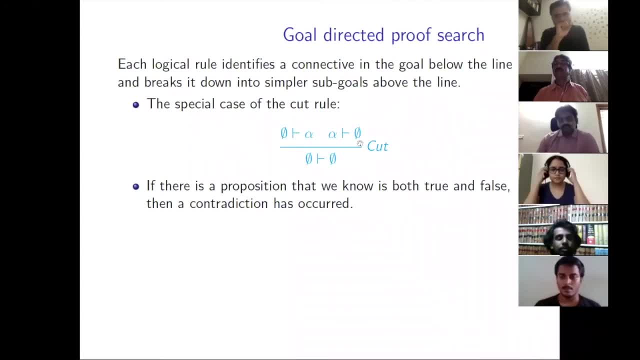 And from alpha you get the empty conclusion. What does that mean? The conjunction of the empty set you think of as true And the disjunction of the empty set you think of as false. So this is: from true I get false. 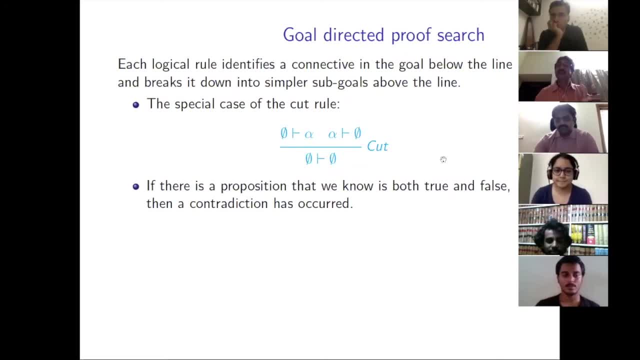 I mean, this is the contradiction. So the empty sequence where you have nothing on the left-hand side and nothing on the right-hand side, you think of as a contradiction. So this is the So, if there is a proposition that we know to be both true, 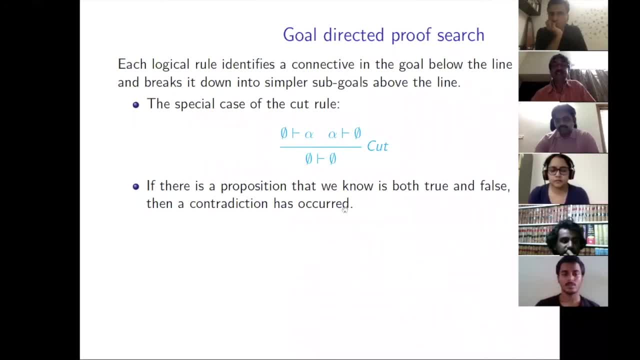 this is what it means: Right It's valid, Right It's false, Then a contradiction. So the cut is actually a way of saying a contradiction has occurred. cut signals in the particular case And the general case, of course, is: 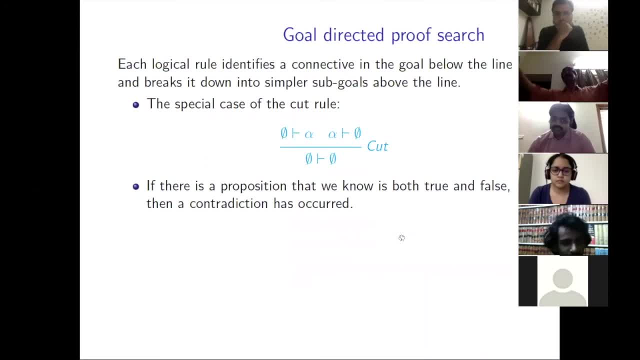 And this is very important because in sequence calculus you combine things from many different parts And in the process you may introduce, And the idea is to discover them, eliminate them And for proof, theorem provers for systems that do proof search. 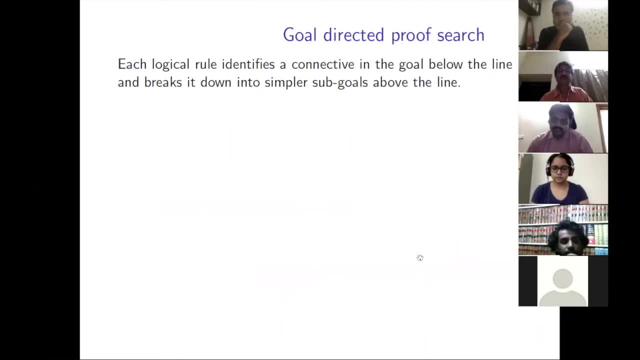 these are, And then something. but I wanted to point this out for another reason. On the other hand, suppose you actually have the empty consequence. I can always do weakening- Remember. I can send in the conclusion and weaken the assumptions, So I can get this as well. 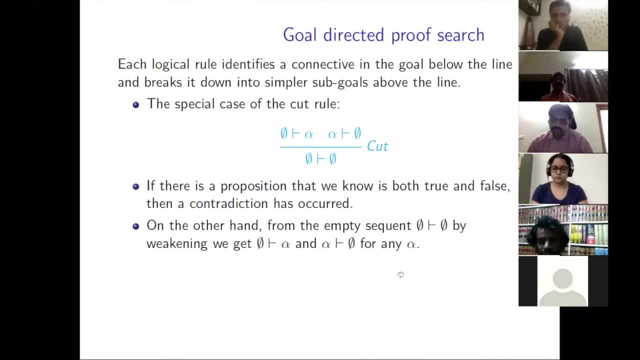 Right. So you can. from these two, from a contradiction, you can get the empty consequence, empty sequence, And conversely, from the empty sequence you can always get a contradiction. So this says that sequence calculus is consistent exactly when there is no proof of the empty sequence. 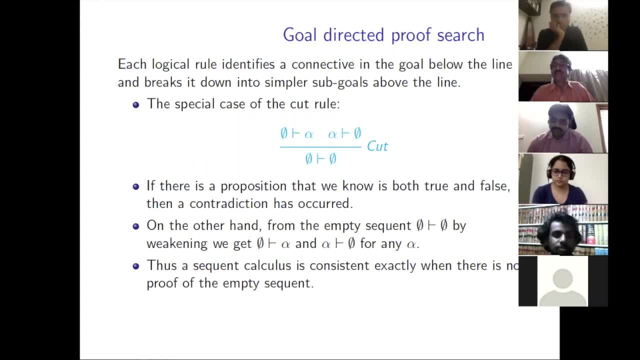 Right. So how do I prove that a sequence calculus is consistent? Well, I prove that there is no proof of the empty sequence. In the case of the Hilbert system, we talked about a set of formulas being consistent. if you cannot derive a contradiction, 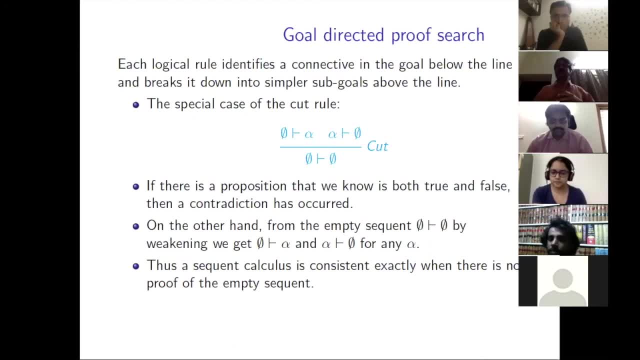 from that set of formulas in the Hilbert system. But how do I prove that a Hilbert system itself is consistent? Only by semantic arguments. Right, By showing soundness. Because suppose the system allows you to derive alpha, negation alpha, then alpha has to be a valid formula. 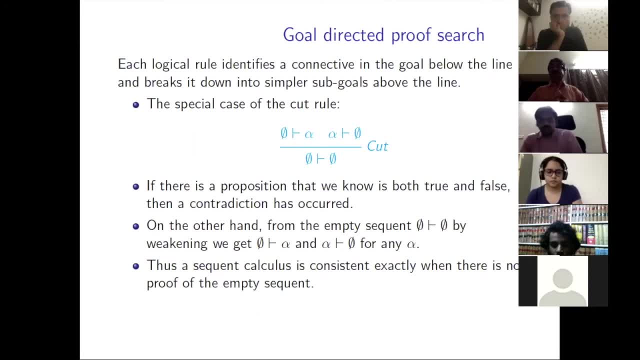 negation alpha has to be a valid formula and that's not possible, Right? So you show that the system under empty assumptions doesn't lead to a contradiction by appealing to models. Now, Genshin was not interested in it, I mean, this is true. 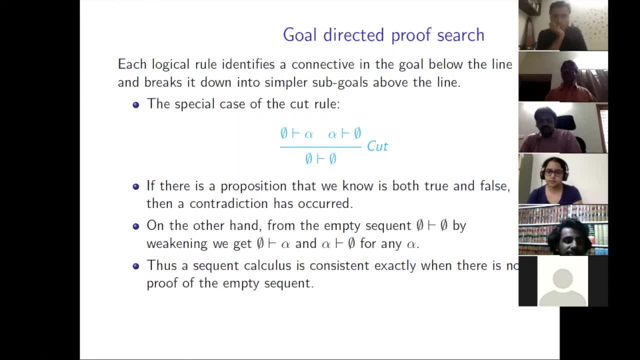 There are no models. You are only talking about derivations, Right? So, and here is the notion of consistency And, as I said, Genshin's entire project was to prove consistency, And he wanted to do it without resorting to models of consistency. 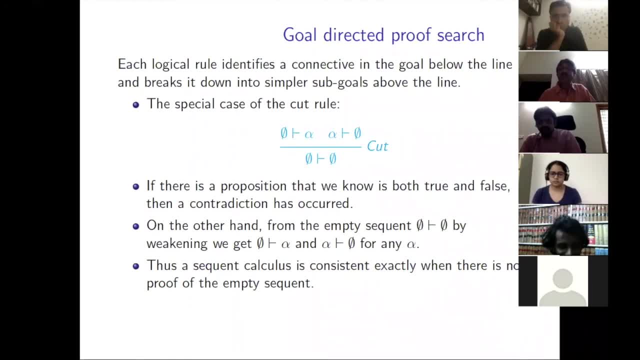 Yeah. So his idea was that you write down some rules, you write down some maxims for numbers and you should be able to show that it's consistent without actually appealing to any semantic structures whatsoever. So in any sequent calculus, 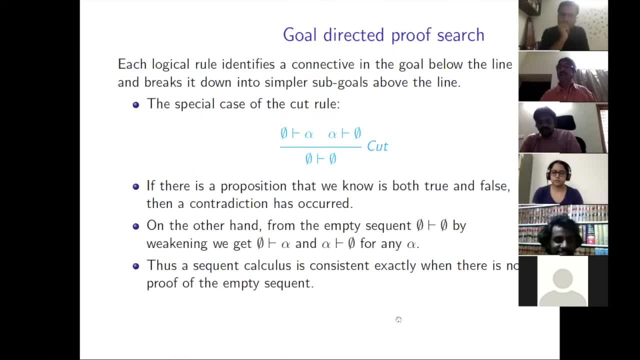 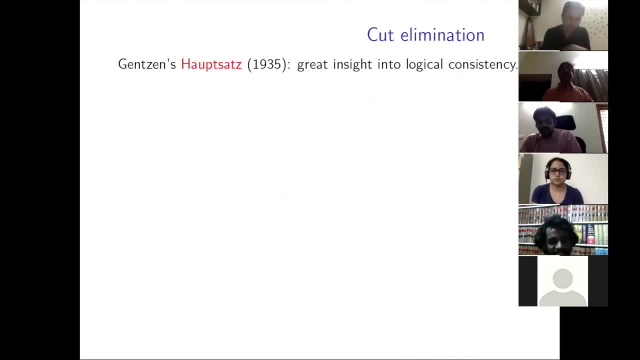 how do you show it's consistent? By showing that the empty sequence cannot be consistent. And in Genshin's 1935 paper, so-called Hopps' art, it's, you know, great insight into consistency. This is the cut elimination here. 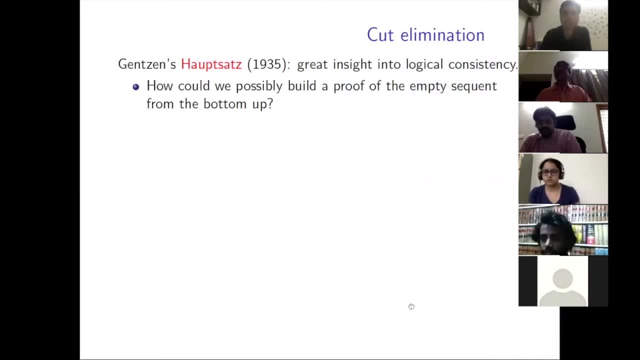 So what is that? So now I want to show that the empty sequence is not derivate. Well, how do you, how could we possibly build a proof of the empty sequence Right From axioms and things like that? 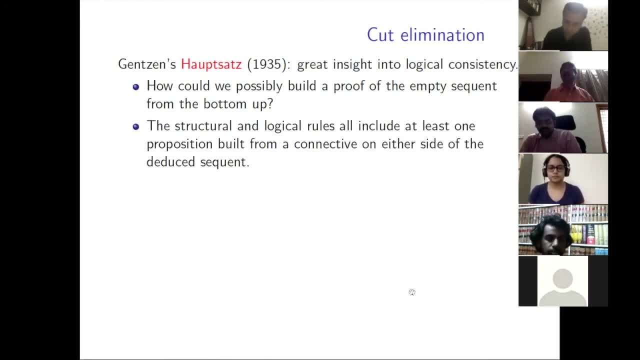 Yeah, Exactly So, if you look at it. and this is where notice that in sequent calculus, everything is using your rules, right, Entirely structural. Now look at the structural rules and the logical rules. All of them will include at least one proposition. 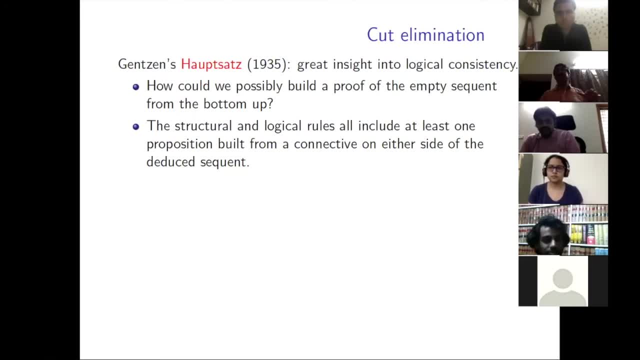 built from a connective on either side of the sequence. So the logical and structural rules cannot give you the empty sequence. If you keep only using logical rules and structural rules, you can easily show that a proof which consists of only structural rules and logical rules. 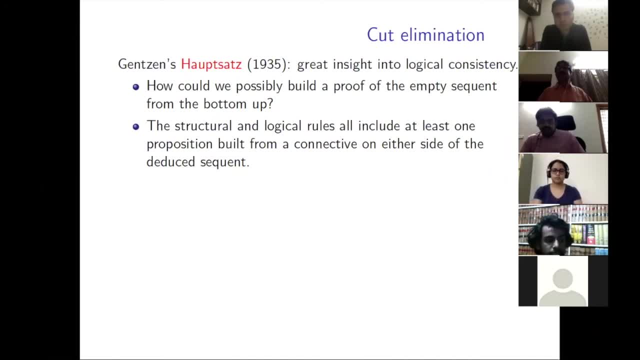 could not derive the empty sequence. This is a routine proof by induction. What about the axiom? Well, the axiom rule just says that if you know, if you have got alpha on the left hand side, you can get alpha Right. 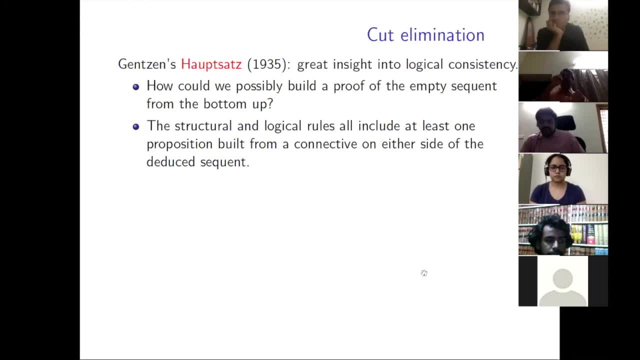 So you can't get an empty. So, using structural rules, logical rules and the axiom rule, there is no hope of getting the empty sequence. So the only inference rules that might ever deduce an empty sequence and therefore lead to inconsistency. 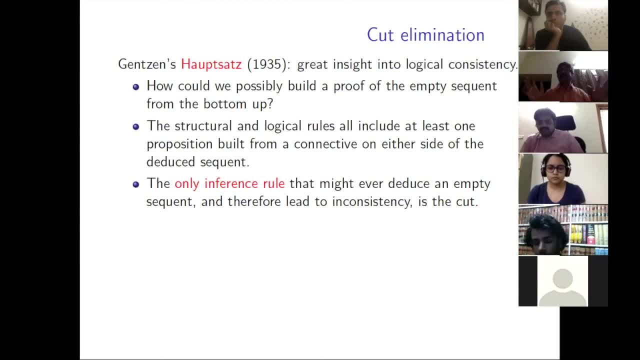 is the curve. And, by the way, if you start doing proofs, you will see it's very easy to do inconsistent stuff because you know you start combining things from very different contexts, which is just, and that's something that 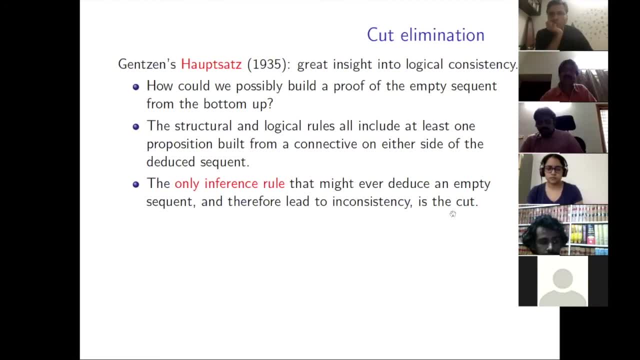 you know you can follow easily. So, and thus the proof of consistency is the same as the proof of the cut elimination theorem. What does the cut elimination theorem say? You give me any proof of a formula that exists, a cut-free proof. 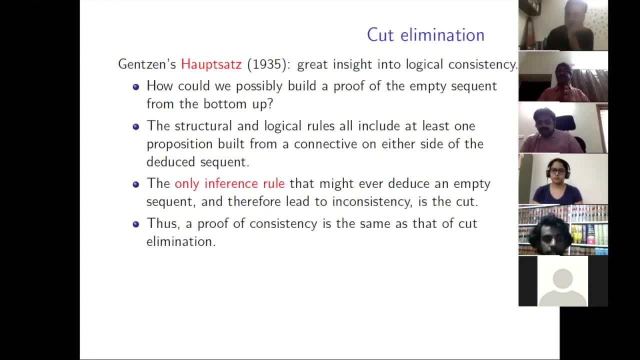 Once I prove this is the cut elimination theorem, What does it say? Take any formula. if it has a proof at all, it has a cut-free proof. If I prove that, and this is where it says- that's all it needs. 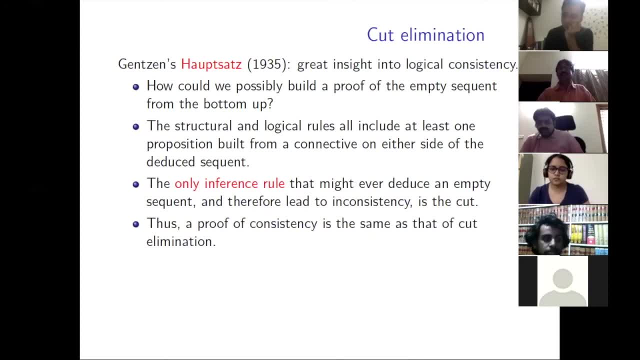 now for consistent. and then he doesn't do it for just the system LK, it's called LK. He doesn't do it just for this calculus, he doesn't do it for arithmetic. He carries out this process for arithmetic. 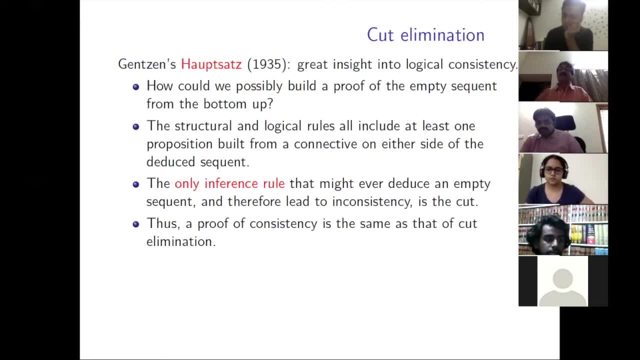 showing that you know the formula is arithmetic right. there's a cut for cut, elimination theorem And there's another very important observation here: Note that the cut rule is the only one that does not have the sub-formula property. 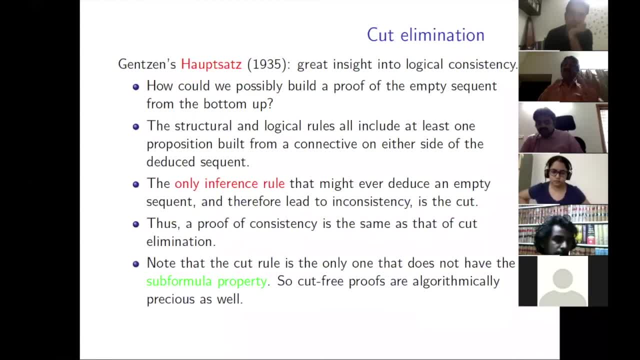 That is what do I mean by sub-formula property. If you look at any rule, if you look at a complicated formula that occurs below the line right, only the sub-formulas of the formula occur above the line. So to conclude, alpha and beta. 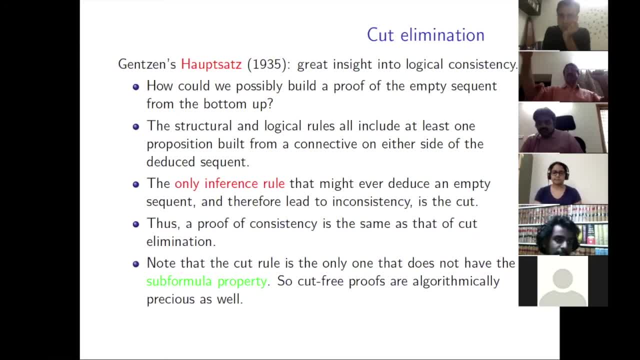 you look at the premises on top, you use only alpha, whatever gamma and delta, Only the things that occur in the sequence below. the only rule that doesn't have the sub-formula property is the factor, Because if you look at the thing below the line, 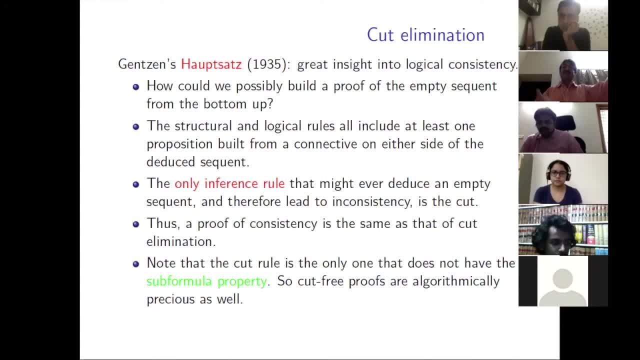 there is no alpha at all. Alpha by magic appears on one side, and So there are two proofs where alpha is So alpha is a formula of arbitrary limit, So for proof-search this is very important. 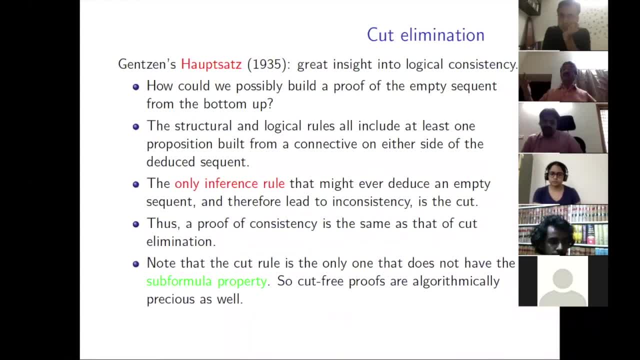 because, if I'm using all, if your system has sub-formula property, in fact, many, many, you know this is something that the observation I have been doing in the cottage industry for many years now for many of our things. 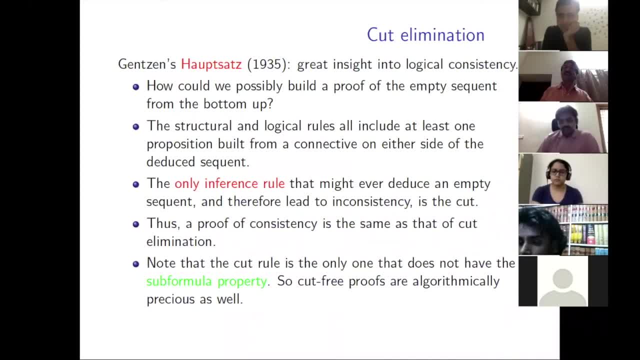 with bounds, using sub-formula property to show that I can do the proof-search in the form of alpha. So, in general, sub-formula property is something sacred to hold on to And they exist. Of course you take a proof. 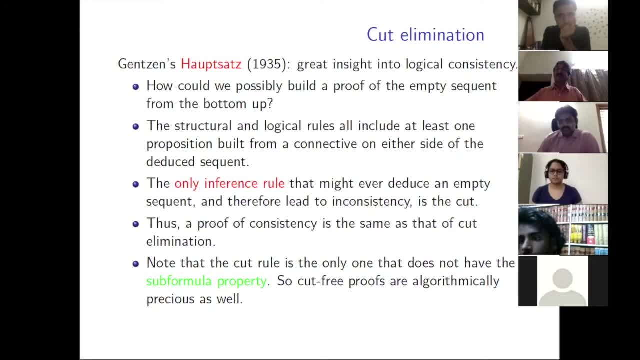 and remove cuts, the proofs may blow up, and that does happen. The cut-free proofs are can be quite huge, But if you are only you know you only have a system without, so sub-formula property is also very important. 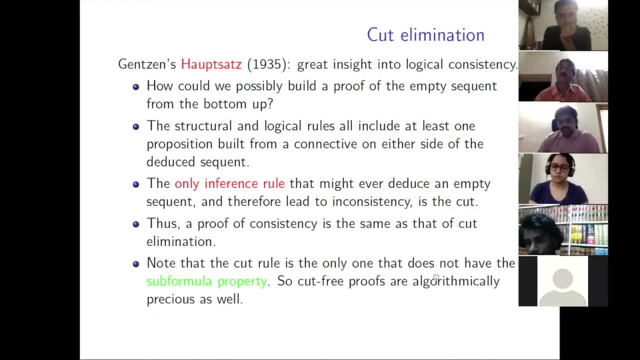 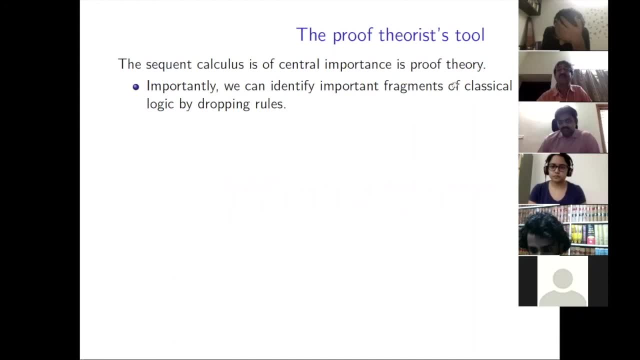 So cut-free proofs are algorithmically efficient, So you can do the proof-search. And the sequence calculus is of central importance in proof theory. Importantly, we can identify many important fragments of classical logic. So, as I said, 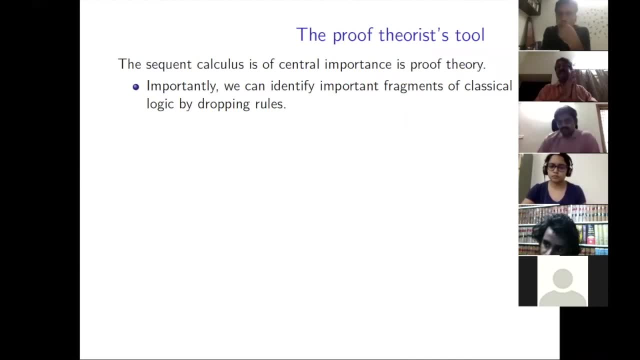 Jensen's interest. he devised this whole thing to prove consistency, But later on, as I said, this has become the main tool of proof theory, and that's because you can look at many, many different things. For instance: 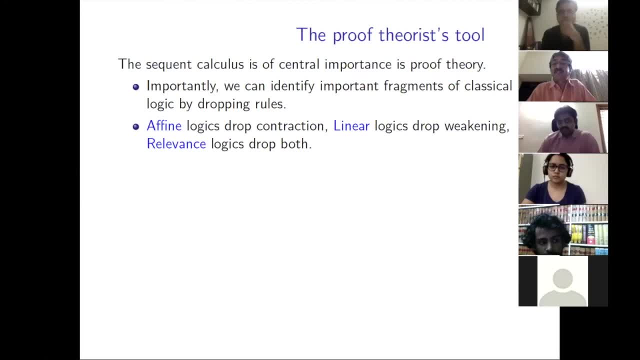 by dropping the contraction rule, you get so-called affine logics. By dropping the weakening rule, you get so-called linear logics, And by dropping both, you get relevance logics. A whole lot of logics are there. 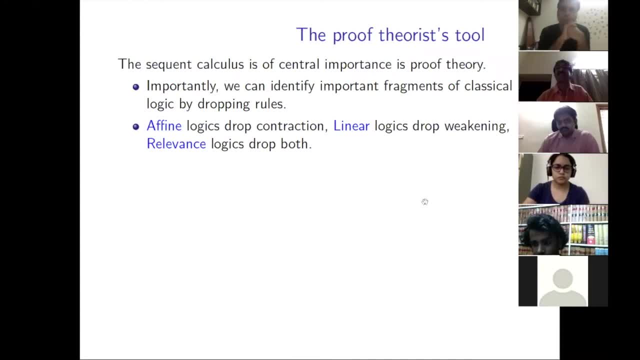 And I'm just dropping names here, I know, but just to show you that there's a lot of insight into this whole structure And then, surprisingly, very small changes in the proof system you receive, For instance, 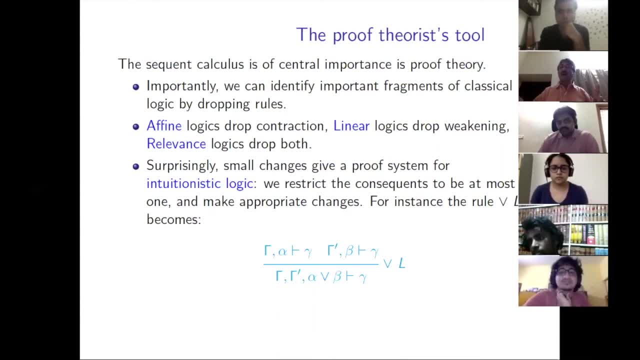 if you restrict the consequence to be at most one, that is, you know it's one-sided sequence: On the left-hand side you have all these and on the right-hand side you have one, And make all the natural changes that you make. 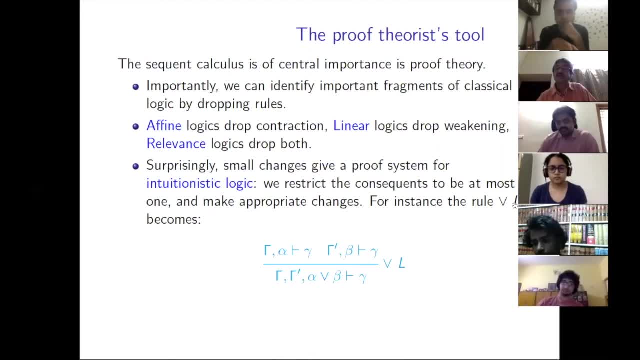 So for instance, the all left rule becomes: well, you have alpha here and you have the gamma. I mean I get the delta And all the rules are. And then you can actually show that. 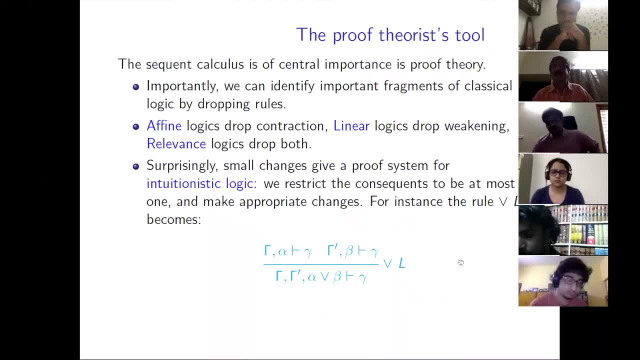 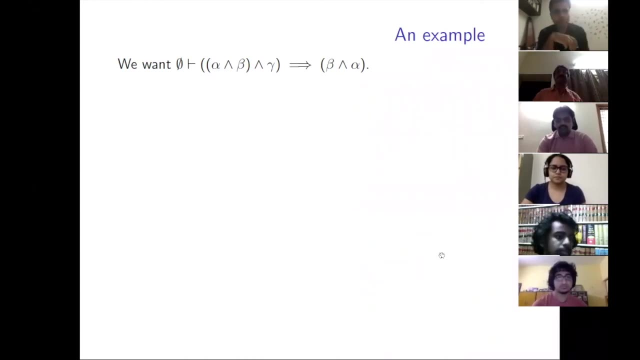 alpha or not alpha is. Can I take another few minutes and show you some examples? Okay, Here is a. I want to show something completely straight forward: Alpha and beta and gamma. This is something of course, it's true. 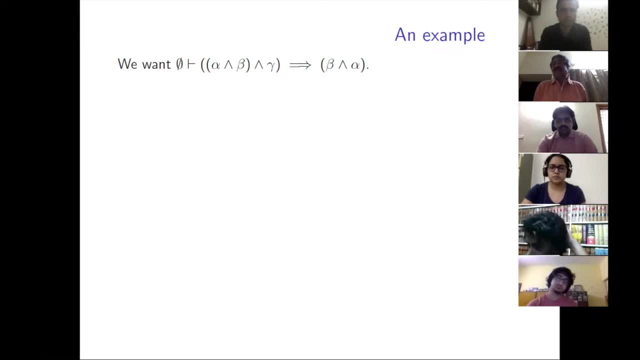 Only to do with the commutativity of conjunction. So you should be using whatever structural rules, conjunction rules And there is an implication. So how does the proof go? Unfortunately, I don't know how to animate. 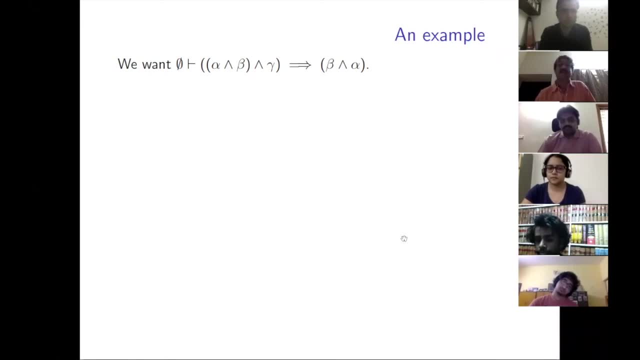 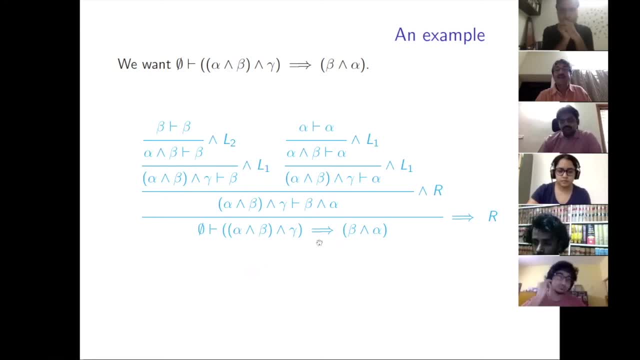 You start from below Right. Now, what is the connective here? The main connective is implication, And I want implication to the right. So the rule you must apply is implication to the right. I mean in SQL calculus. 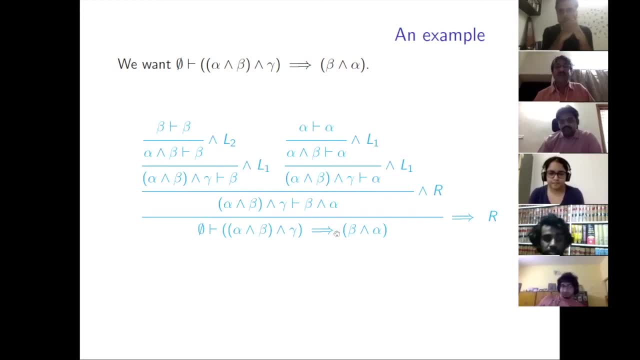 it's exactly this kind of structure. So if I'm using the implication rule to the right, how did I get the implication By pushing the assumption to the left and the conclusion to the right? So do that. So what I want is: 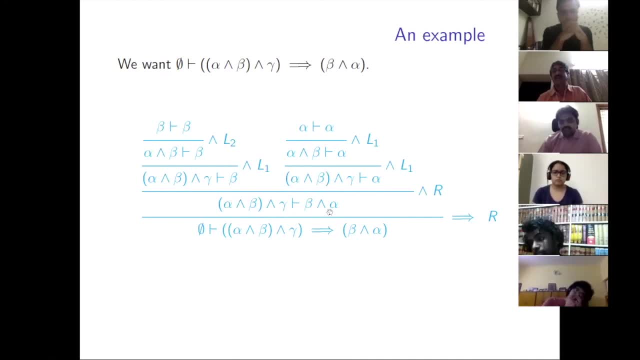 the sequence alpha and beta and gamma to the left and beta and alpha to the right. Well, I've got a conjunction to the right hand side. So what is the rule that I apply? The conjunction to the right That says: 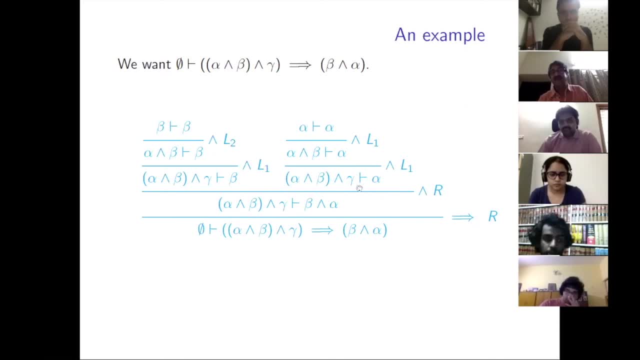 from this assumption: if I've got a beta and if I've got a gamma alpha separately, I can combine. So push it up. Now, how do I derive this? Well, I've got alpha and beta and gamma. 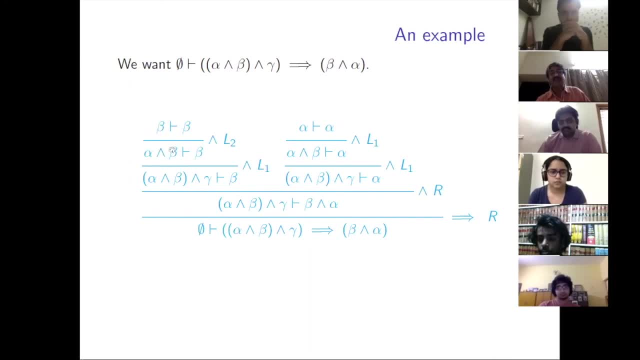 So by left rule it suffices to get only alpha and beta, And then by left rule two one here. you can see here that beta has been we. you know we can. we can get the assumptions. 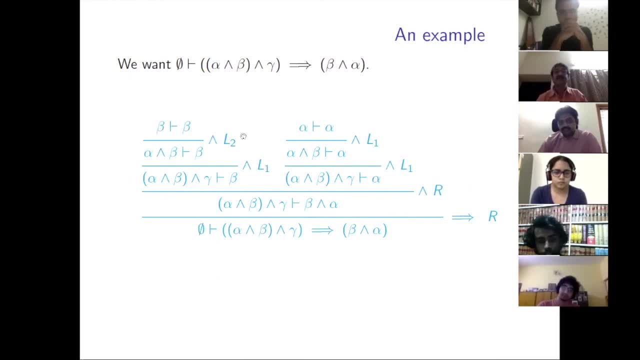 simply So, that's all. So either you start from, but the thing is you can never do bottom up. You could start with the answer and then say, ha, here I can send them, you can. the assumption. 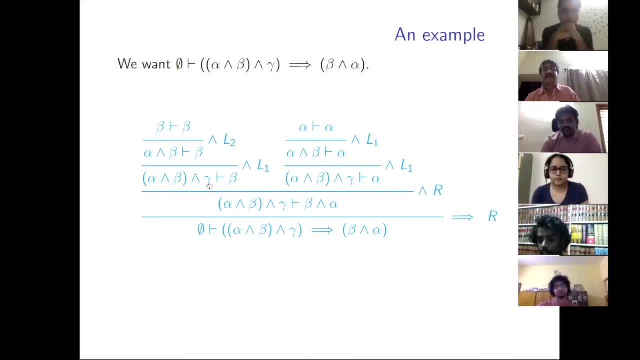 beta here I can, and then I can add a gamma inside And from that you know you can combine. But, as I said, this is not how it goes. It's goal-directed, it's a deep search. 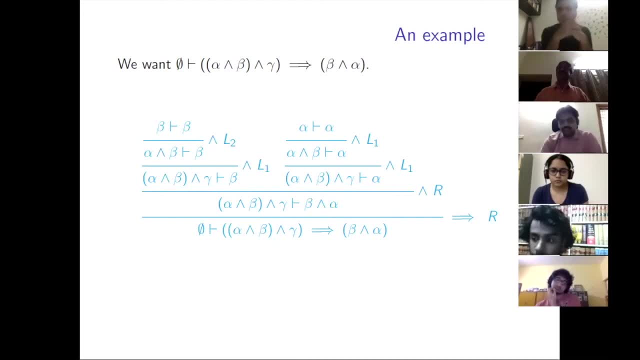 You proceed the other way and the rules pretty much take you to the axioms, Decompose things into smaller and smaller sub-rules, Here so called law of excluding. And how does the proof of 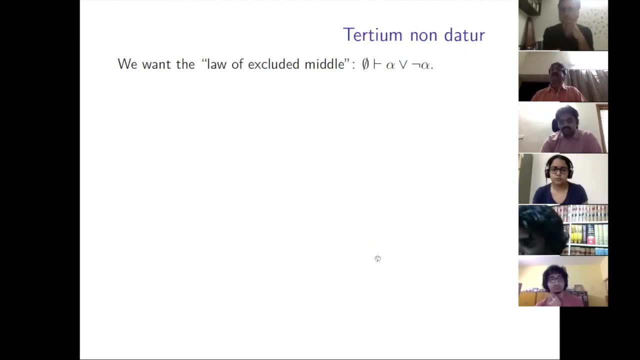 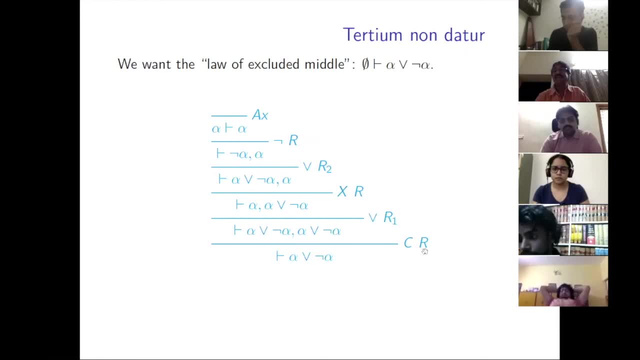 Here I have used the contraction. What is the contraction rule? I just make two copies right, And in the two copies I have used the OR-rule to the right. So this is beginning from alpha. 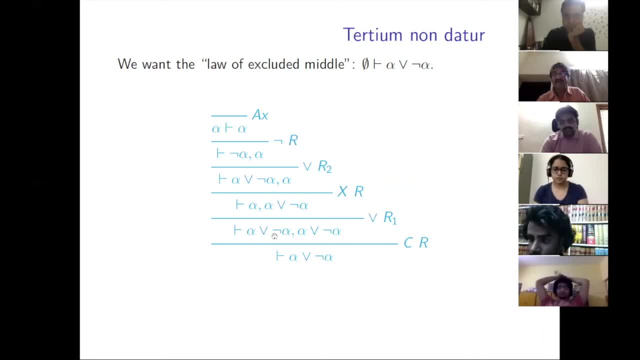 and then I have moved to alpha, OR-rule, And then I use, exchange, push these two And I make like this first successes And and now again I use. so I've started with not alpha, and then negation rule says I: 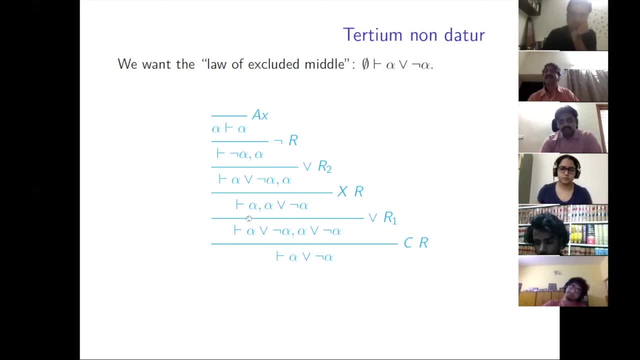 can push it inside again. it's clear then, some engineers, how did this first step happen? how do you come up with the fact that you are actually? but this is only to point out that not only are there are logical rules, the structural rules also come in you and you have to use the structural 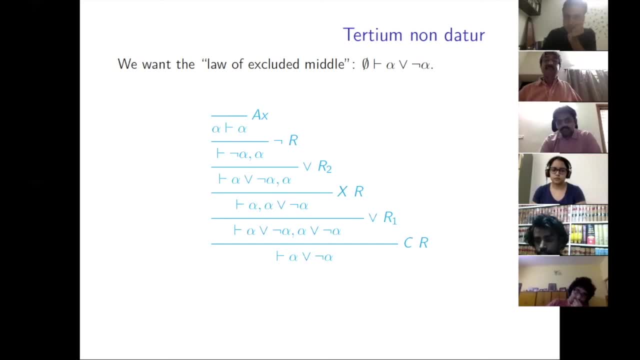 structure, Because the logical rules are very specific. They apply only to the leftmost or the rightmost and then to the left disjunct or the right disjunct, or left conjunct or the right disjunct, And therefore to get whatever you want to do to that position, you have to use, for instance, 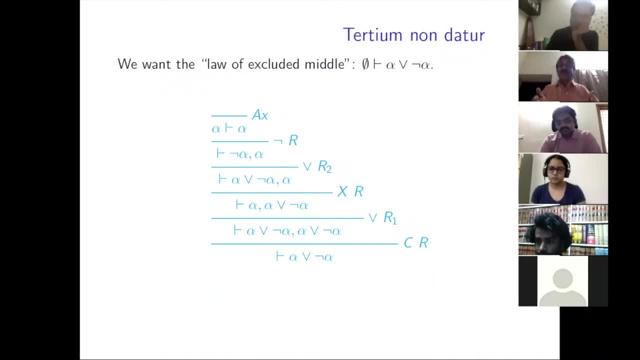 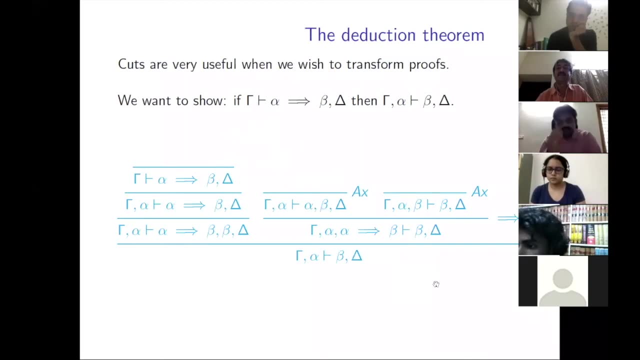 exchange and you have got only one formula. you need two formulas, all that kind of things. Another example, and this is to show how cuts are actually useful. Now remember that in the Hilbert system, the non-trivial part of the deduction theorem was this way: 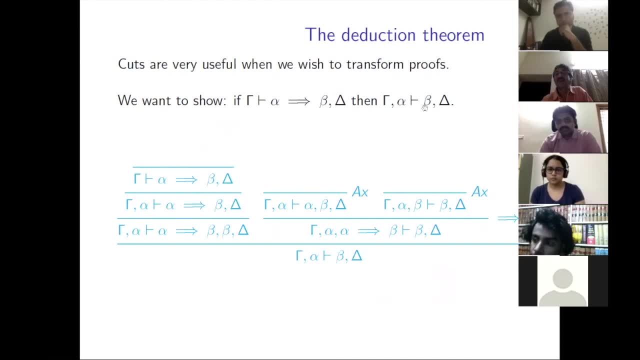 Trying to show that if gamma union alpha derives beta, then from gamma. there is a proof of alpha implies beta. In fact I did a proof by induction and introduced the axioms in the process. Now I don't need that in a sequent calculus because that's in fact the rule for implication. 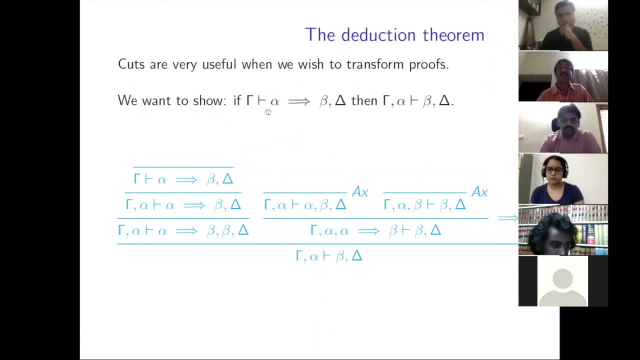 So, whereas the other direction is non-trivial, if from gamma I have derived, alpha implies beta, then gamma with the assumption alpha I can derive. How do you do that? Well, this is what I do. What I do is I use the cut rule. 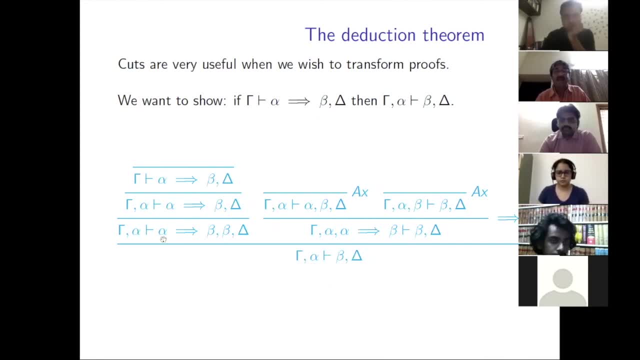 Since I have got gamma, alpha and beta delta, I put in an- alpha implies beta to the right hand side here and alpha implies beta to the left hand side here- and use: cut. Now how do I, for instance here, you can see how do I have an implication on the left hand. 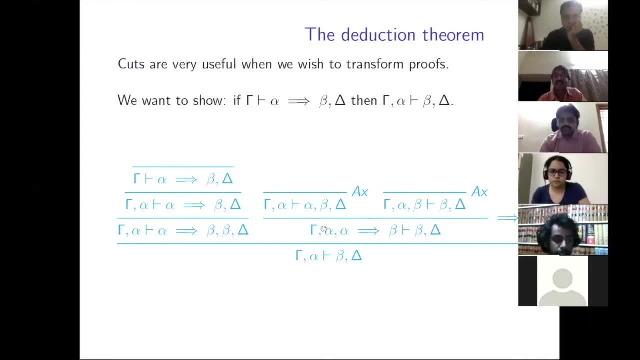 side. Well, an implication on the left hand side means that I should have the beta on the left hand side and the alpha to the right. and well, let's start right now, and I see that the axiom will be just like this: from beta to the delta. 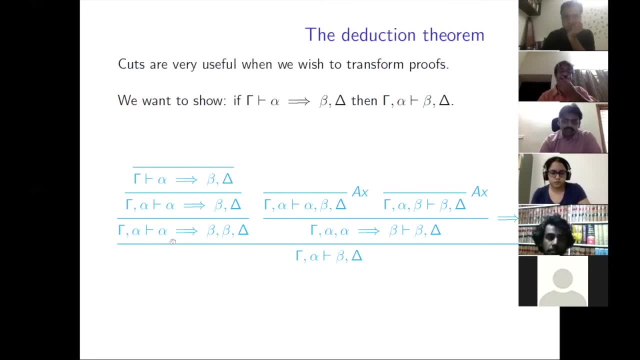 So what about here? Yeah, Yeah. So here, I first weaken it and I use weakening to get rid of this multiple alpha mass, and then I bring it down to form, which is what we had. We had this and we want to show this. 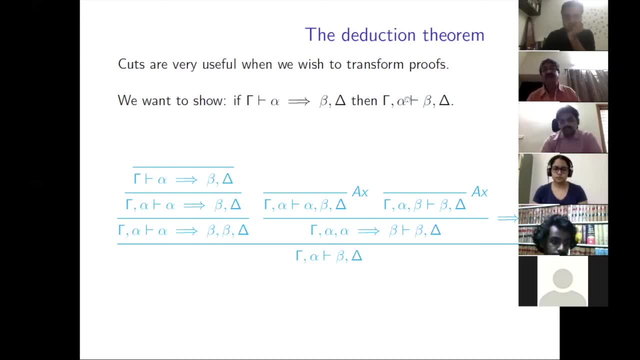 So this is some proof that you are given on top of the proof you are building up. Okay, let me repeat what I always say: Right? So these kind of formal proofs- it doesn't matter whether it's a Hilbert system or natural deduction or sequent calculations- by watching some, least of all- at least if I was doing- 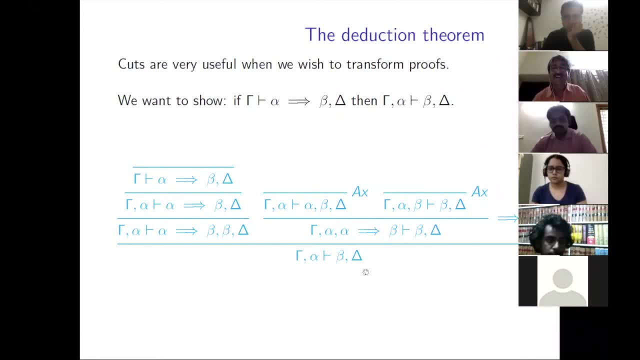 it on the board. I would actually start with this and do it slowly, Fortunately in slides. that actually is not presenting the finished proof to you, and I know that there is no hope of understanding the finished proof by just looking at something, So the only real way is to work it through yourself. 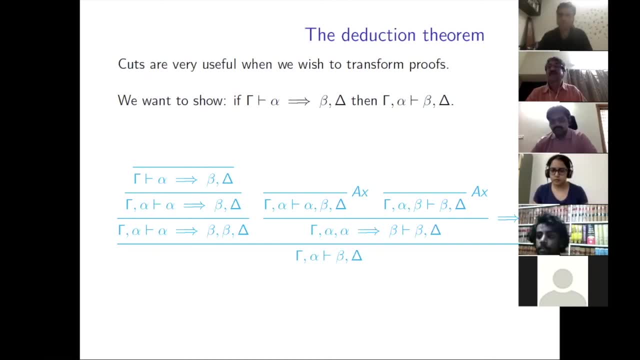 But these files will be with you and I can give you the results. So the thing is that to actually get used to doing these things, so of course I would say, do some exercises or doing some of the things, and we already had a bunch of examples. 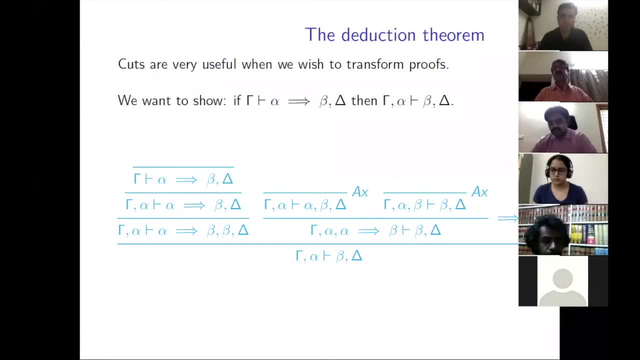 for the Hilbert system, Natural deduction. I think I did, But for simple propositional formulas. if you try out, dirty your hands see how all these play out. Yeah, That's it. Any questions? Okay, Thank you. 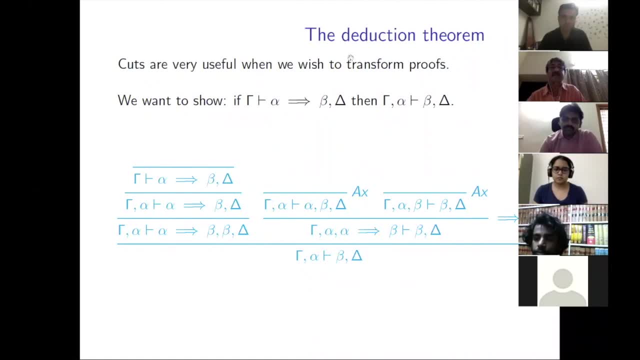 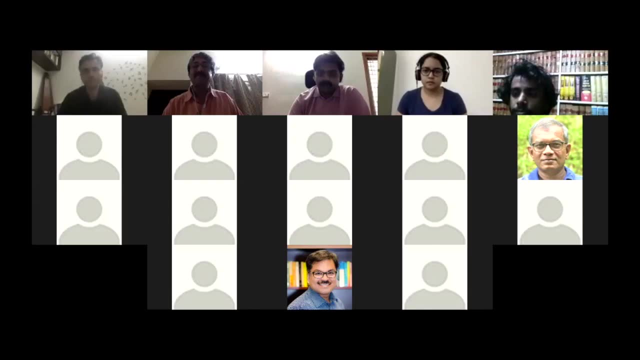 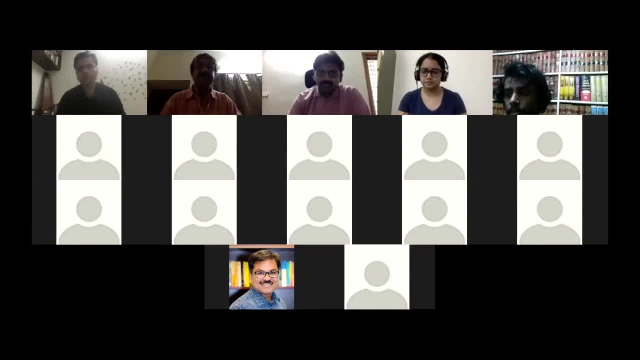 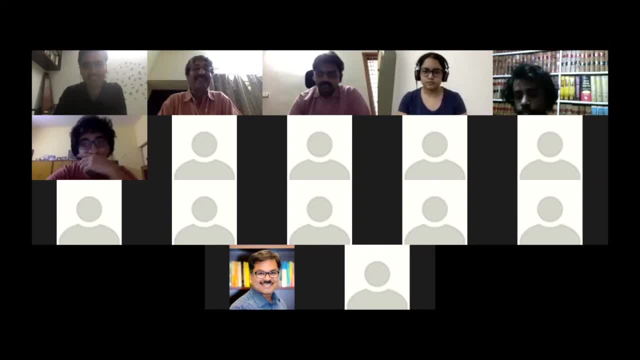 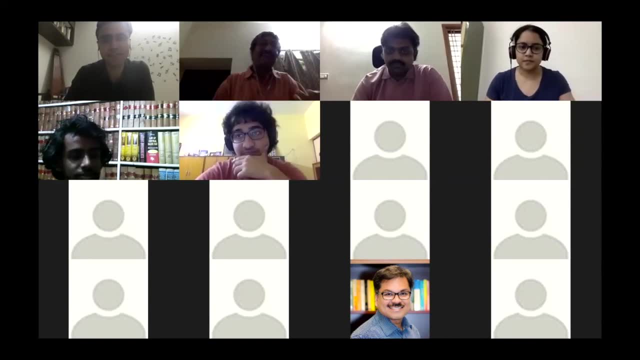 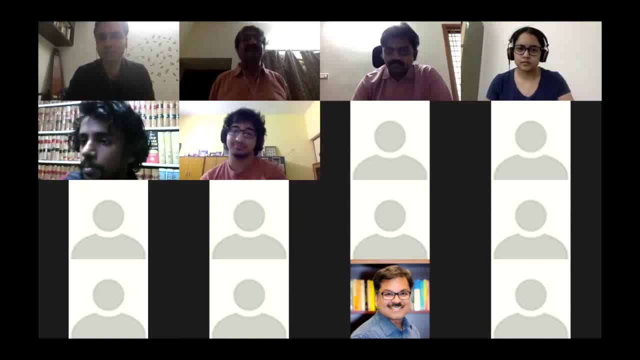 Unfortunately not. As I said, in the process of eliminating a cut, you always blow up So you can prove that that's not a lie. I mean, otherwise this would be. I mean, this is propositional logic. PNP question is floating around. I mean, not in this particular case, it's the NP co-NP question that's floating around. 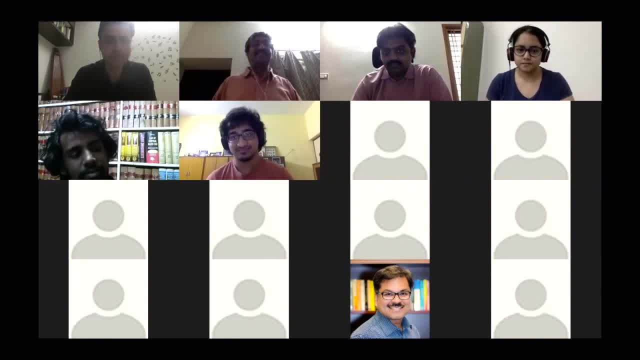 If you're doing proof search, you're actually looking at precisely that question, So there is no easy answer to that. Thank you, Yeah, but as I said, I mean, remember this is 1935, right, So Genshin's insight into propositional proofs is something remarkable. 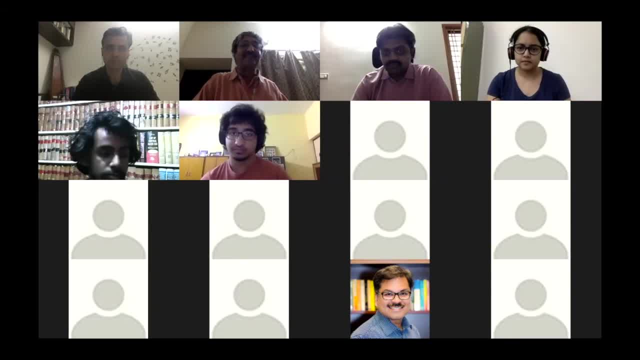 And after what? all this time we are still struggling with propositional proofs, right? They have no clue. We don't know the status of PNP And of course you know Genshin was interested not in, just in propositional logic. 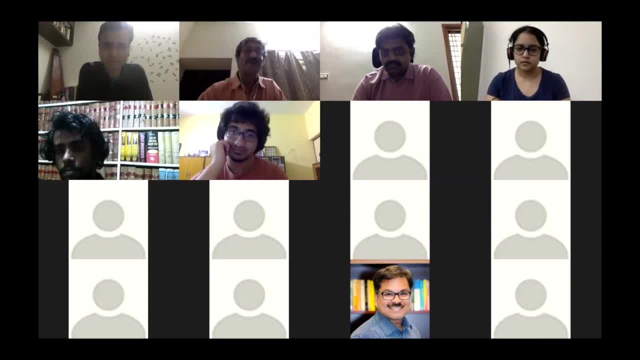 He was interested in, not in, first-order logic. So that's all, Yeah, I mean. second, calculus is particularly interesting if you look at things like linear logic. As I said, what does it mean to drop this weakening rule or contraction rule? 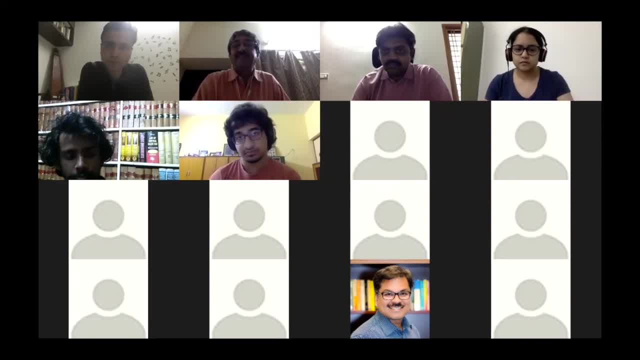 What does that mean really? Like in case of linear logic, formulas don't represent truth values. What it does is, you know, alpha and beta are not truth values, not of a true and false. It's a whole cake. Having two cakes is not the same as having one. 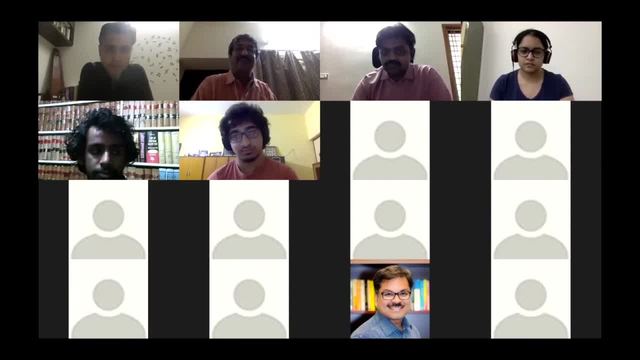 You make identical copies of two alpha. alpha is not the same as having alpha, So that's why weakening is not allowed. Yeah, weakening is not allowed. So from alpha you can't derive alpha, So it's like making copies. 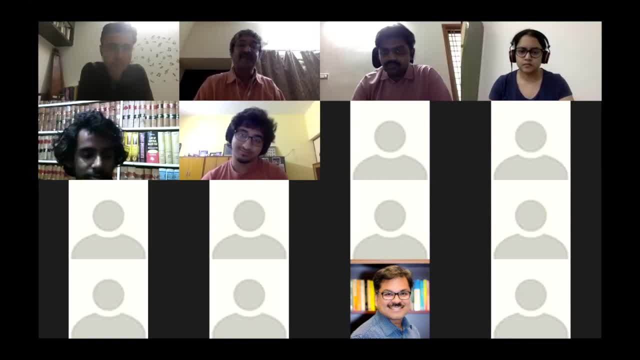 So he calls it a resource-conscious logic. So this is just to point out that if you were to think of deduction as computation, these things matter like hell. After all, you have to write down your formulas somewhere, these things somewhere.